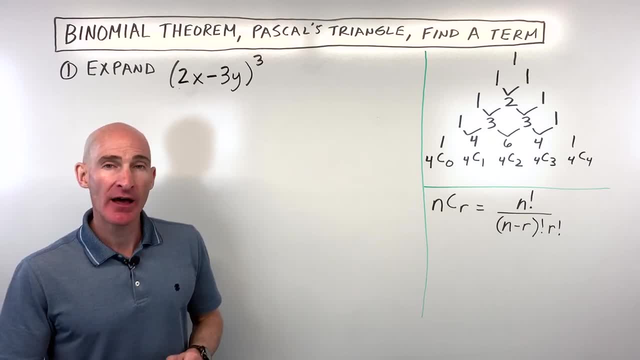 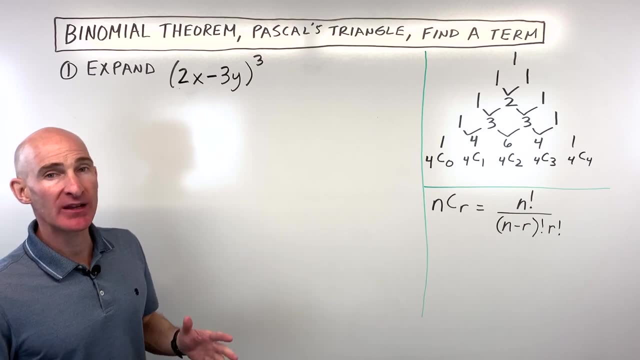 coefficient. So we're going to go through six problems. I'll have some that you can practice on your own. We'll go through all these together and I'll show you some tricks and techniques as we go through this, just to pay attention to. So let's start off with this first one, If we want. 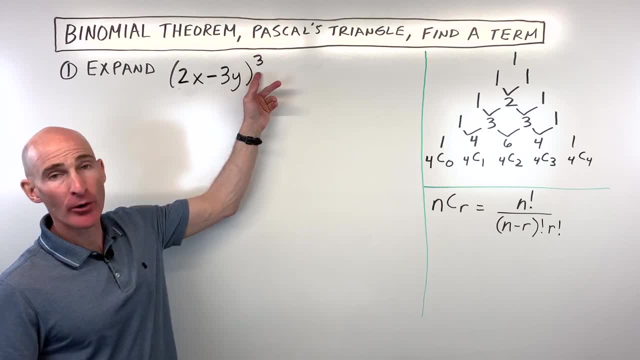 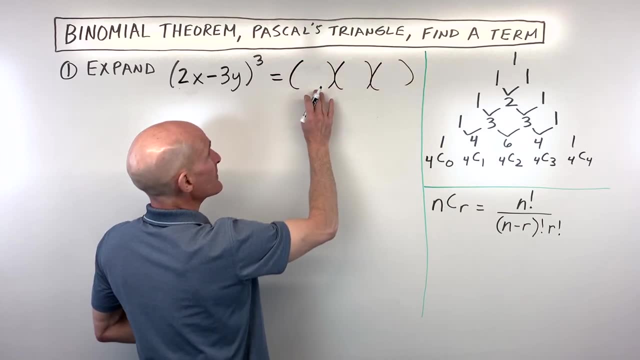 to expand 2x minus 3y to the third power. one way we could do this is we could just think of 2x minus 3y multiplied three times, So we have three of this group. We'd have to FOIL two of. 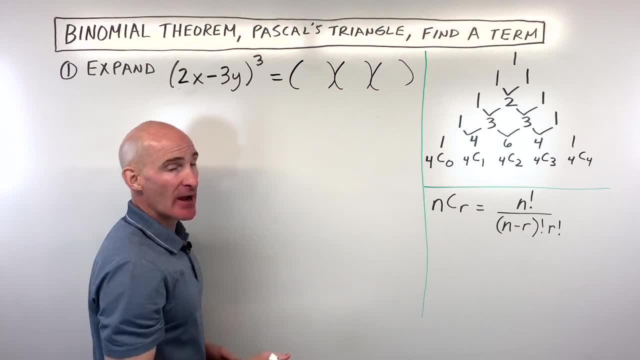 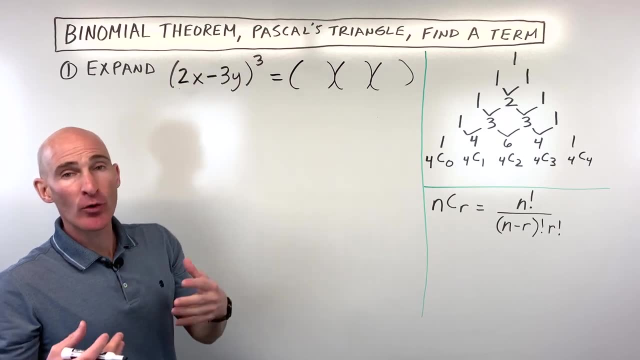 these together, multiply them together and then multiply by this last binomial and then simplify. So that's one way to do it. but the binomial theorem is designed to make this a lot quicker, especially when you raise this to like a higher power, like 4 or 5 or 6, etc. So what we're going? 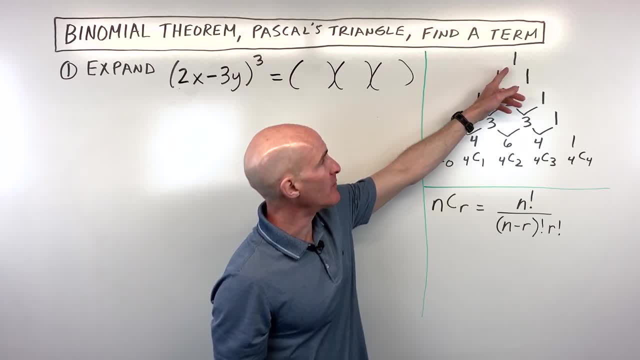 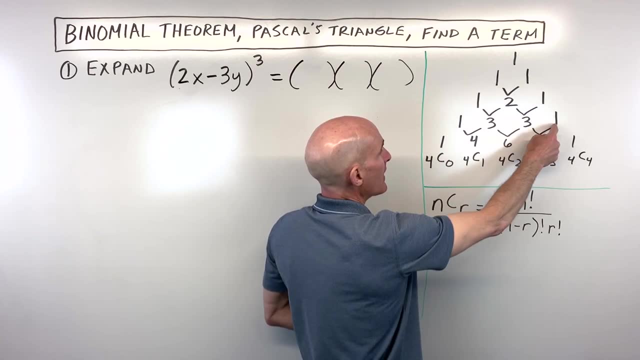 to do now is we're going to go into more detail about this and we're going to start with the going to do is we're going to talk about Pascal's triangle and Pascal's triangle, basically it starts with one and each row starts with one and ends with one. Okay, you can see that. and then what? 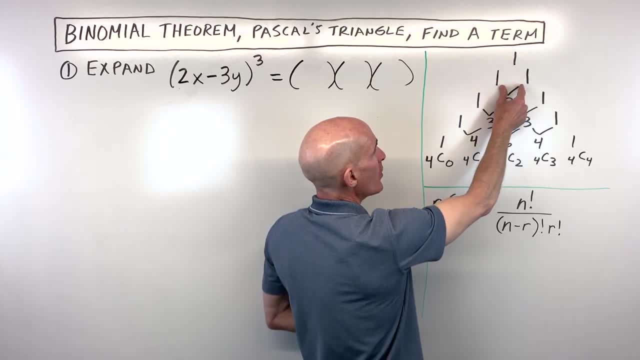 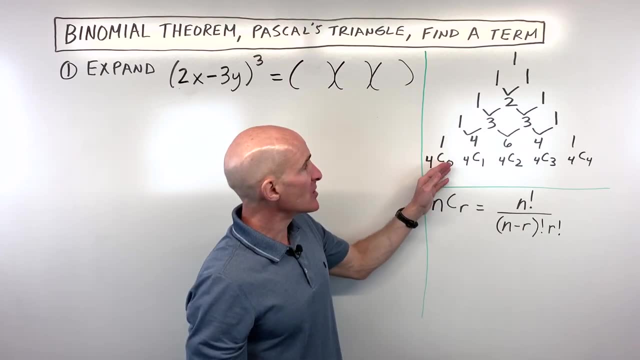 we're doing is you're adding the terms above it to get the term below it. So one plus one is two, or one plus two is three, or etc. and you keep working your way down. But where these numbers can also be derived from is from the combinations. So when you learn about permutations and combinations, 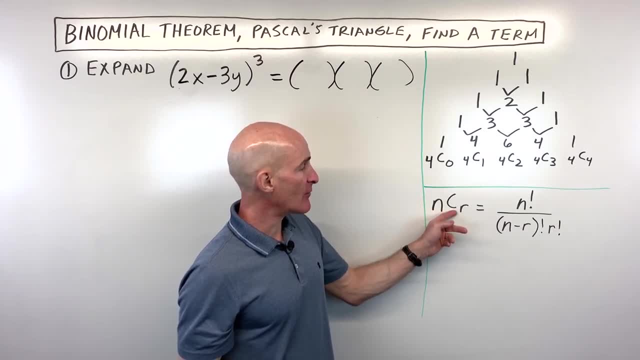 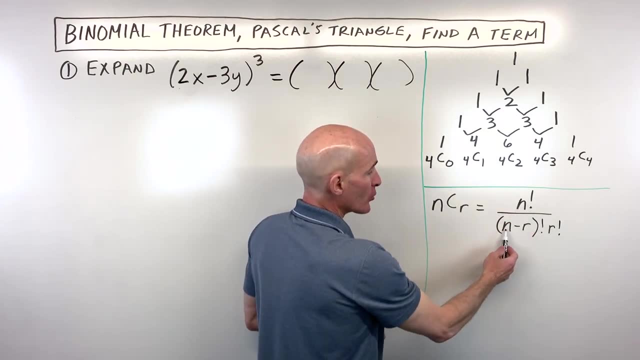 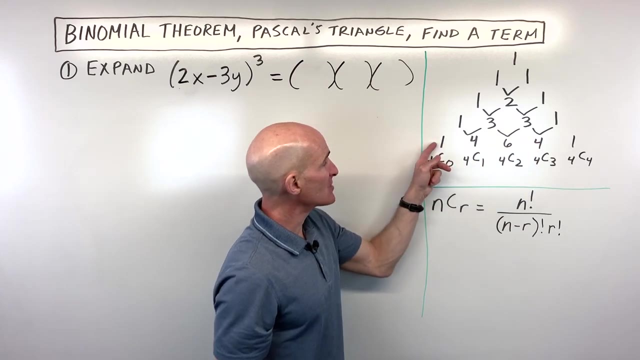 remember the ncr out of n items, how many ways are there to choose r of those items where the order doesn't matter? and we use this formula: n factorial over n minus r factorial, r factorial. So what you could do, let's say, for example, if you're down here at this row, okay, which this is called the fourth. 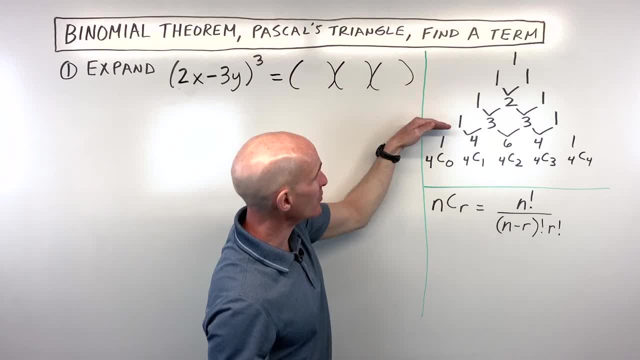 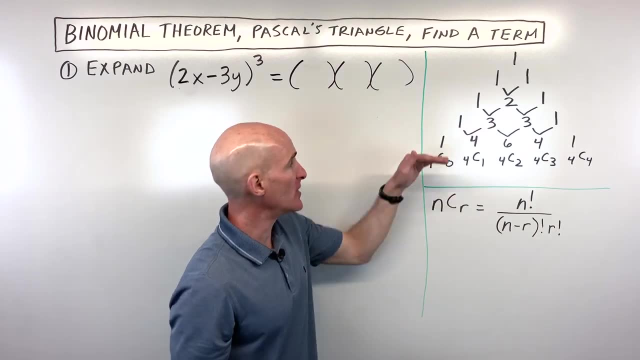 row. it starts at row zero, then it goes one, two, three, four. You can tell what row you're on if you just look at that second number. see, this is the fourth row or the third row. that's the one way to kind of help as you go further down. 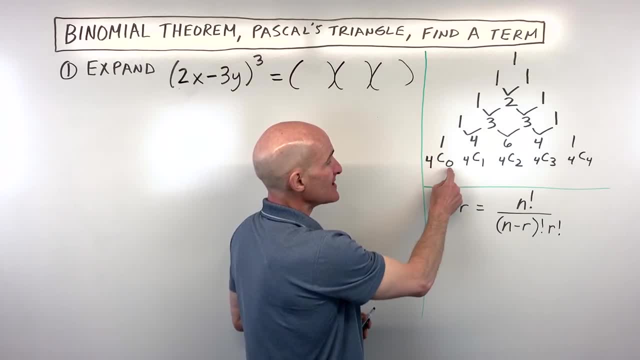 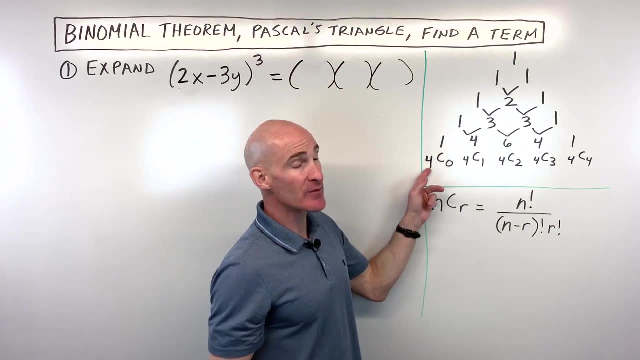 But this one here really comes from four c: zero out of four items. how many ways are there to choose zero where the order doesn't matter? Well, there's only one way of choosing zero items out of four. right, and then this one out of four items. how many ways are there to choose one item where? 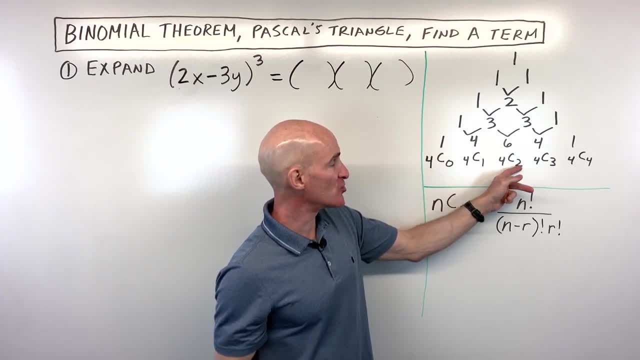 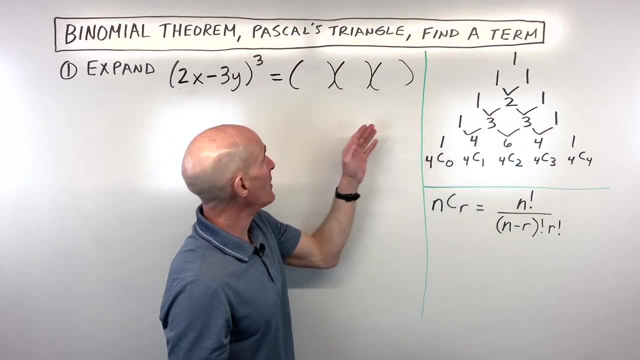 the order doesn't matter, that's four. and out of four items, how many ways are there to choose two? where the order doesn't matter, that's six ways, etc. But what we're going to do is we're going to use these coefficients to help us in this expansion here. So what we can do this: 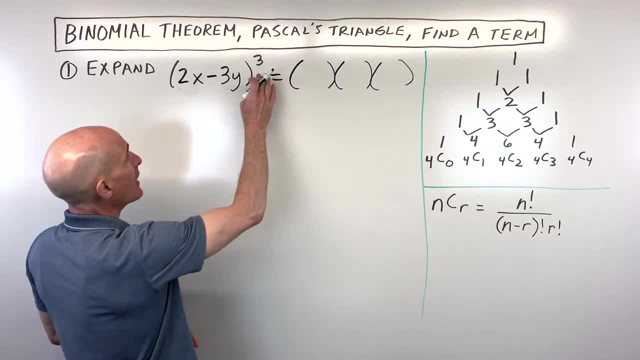 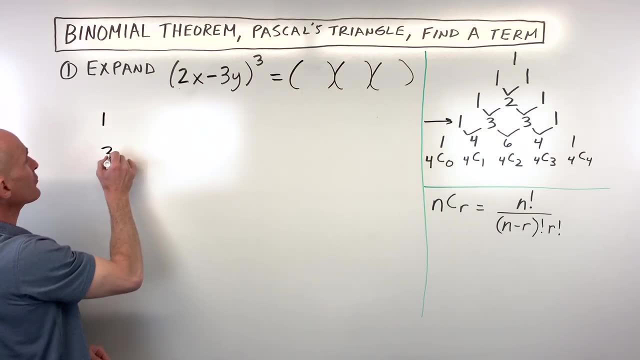 a couple different ways. one way to do it is to start with. this was to the third power. so we're going to start with row three here and these are going to be our coefficients: one, three, three and one. Now remember where these come from. this is really the same thing as three c zero, three c one. 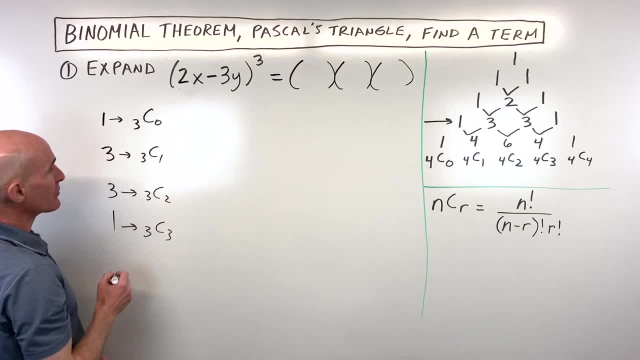 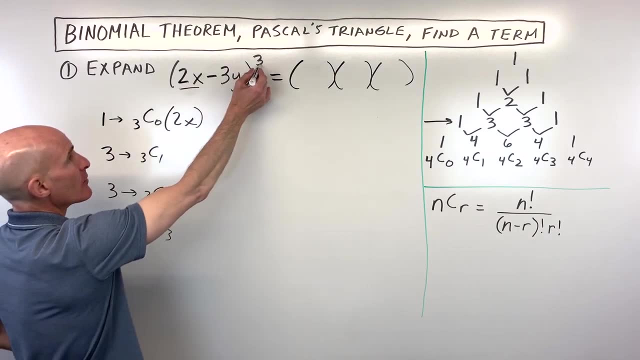 three c two and three c three. Then what we do is we take this first term, two x. you want to take that whole group here And you're going to raise it to the third power and then you're going to go in descending order. so two x to the second. 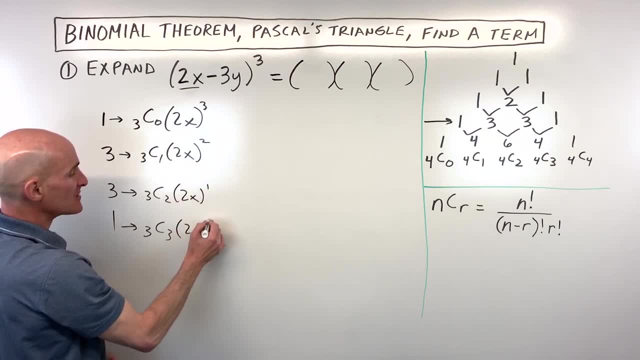 Two x to the first, two x to the zero power. Then you take the second term and you want to make sure you capture that minus sign, that negative sign. This is going to be negative- three y to the zeroth power. and then we're going to go in ascending order. 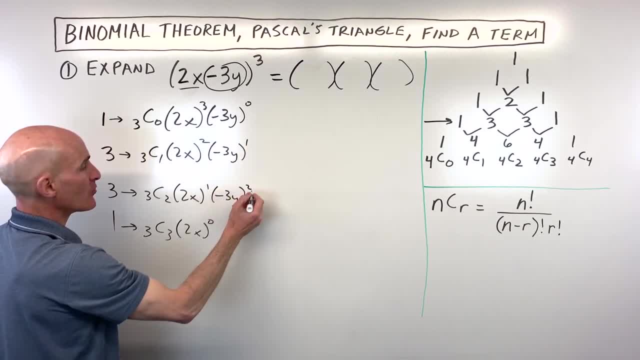 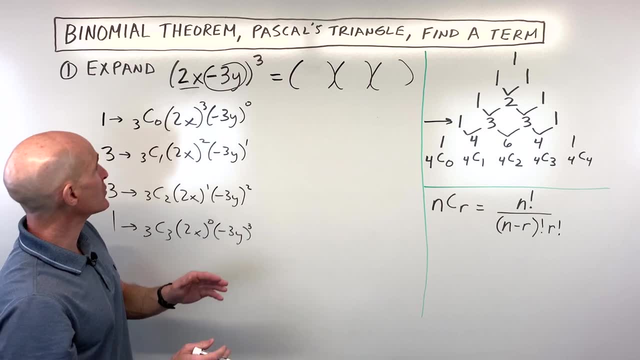 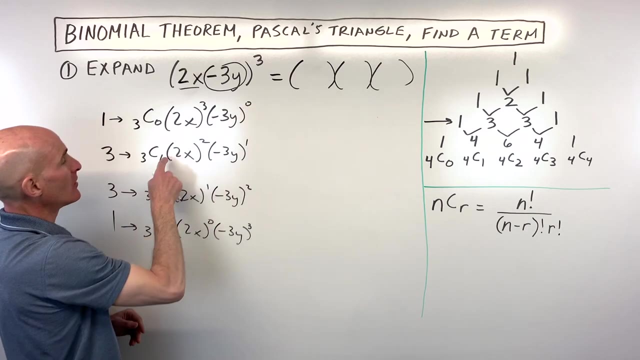 So we're going to go up. so negative three y to the first, negative three y to the second. negative three y to the third. Now I want to show you some patterns here that are important to recognize. Notice how this r value, zero, matches the second term's power here, zero. See one one, two, two, three, three, that's. 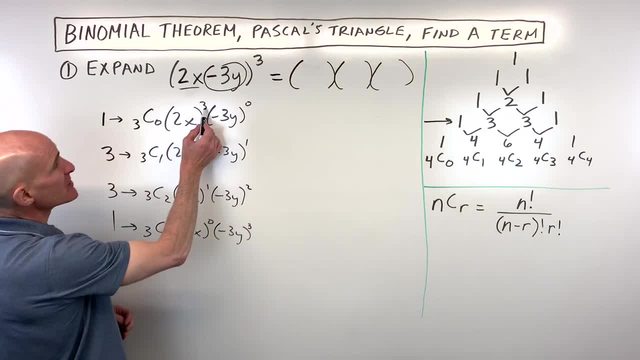 important. we're going to use that a little bit later in this video. The other thing that's important to remember is see these two exponents: three plus zero is three. two plus one is three. one plus two is three. zero plus three is three. Now what we're going to do is: 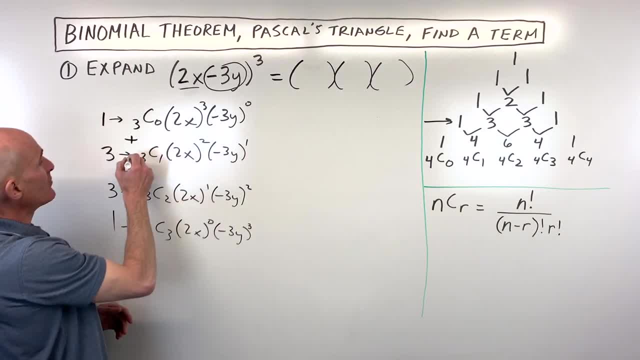 all these are terms are going to be added together, so just think of a plus sign between all of these terms. Let's go ahead and simplify. so we have three c zero, which is one times two x to the third power. So this is coming out to one. 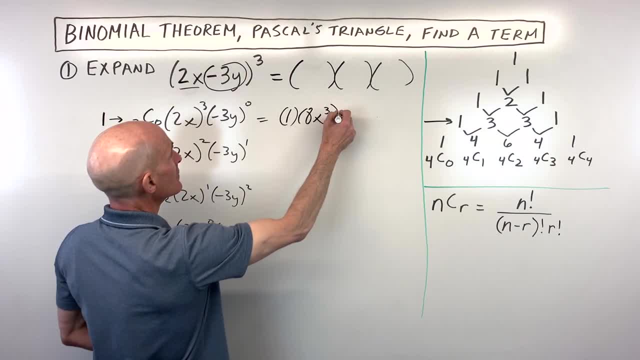 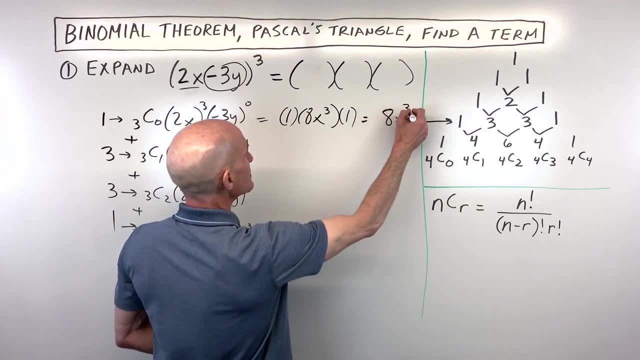 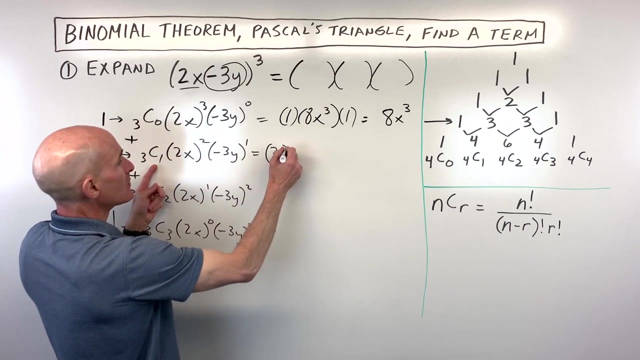 two cubed is eight, so this is eight x cubed, and anything to the zero power is one, Okay. so if we simplify that, this comes out to just eight x. to the third power, Okay. the next term. we have three c one, which is three. We have two squared, which is four x squared. 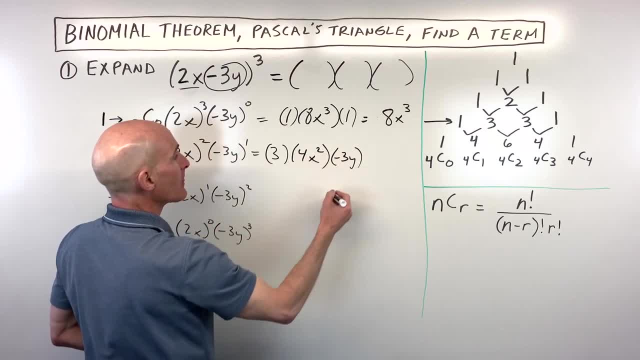 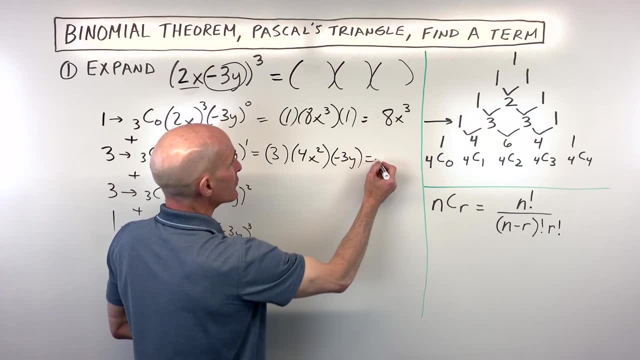 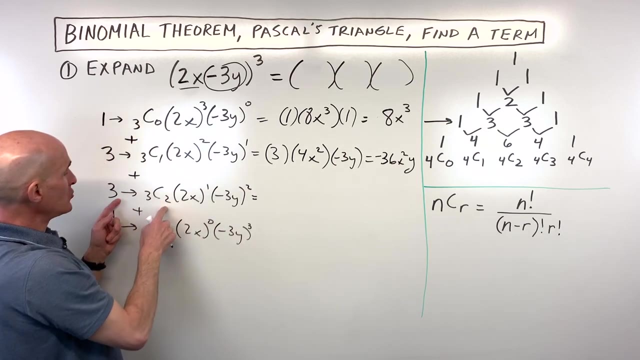 Negative three: y to the first. of course, anything to the first is itself. And so now, if we simplify this, we get, let's see, negative nine times four is negative. thirty six x squared y. Okay, and then for this next term, we've got three c two, which is three. 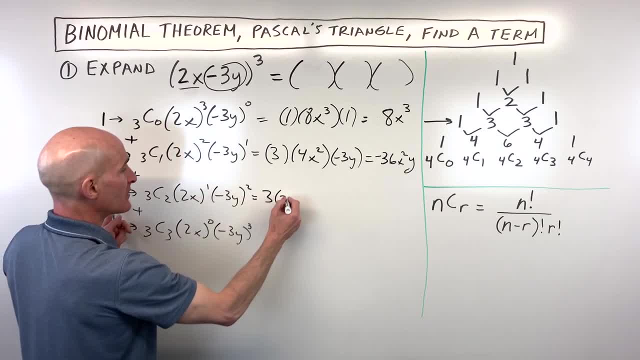 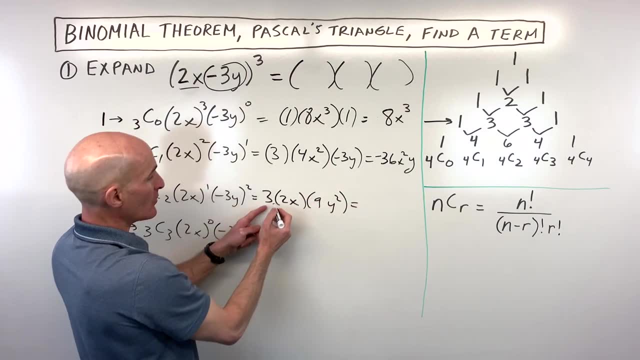 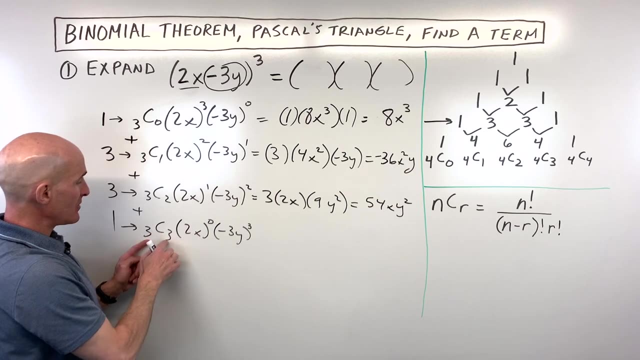 And we have two x to the first. anything to the first power is itself Negative. three squared is nine, y squared. Okay, so if we simplify that, we get six times nine is fifty. four x, y squared. And then the last one, three c. three is one and anything to zero. here is one. 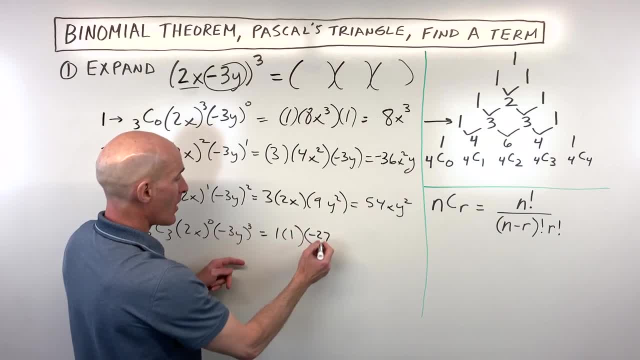 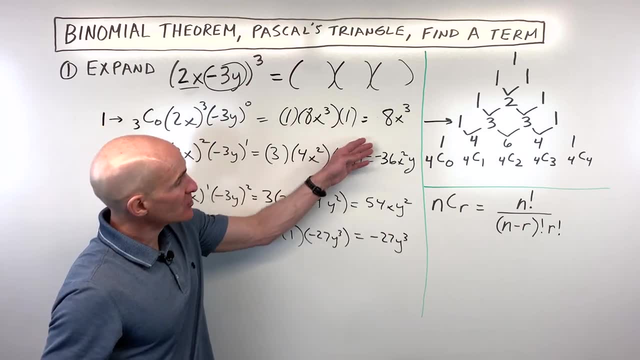 And then negative three cubed is negative twenty seven y to the third power. So if we multiply all that together we just get negative twenty-seven to one cubed. So all these terms are going to be added together, so our final result is going to be 8x. 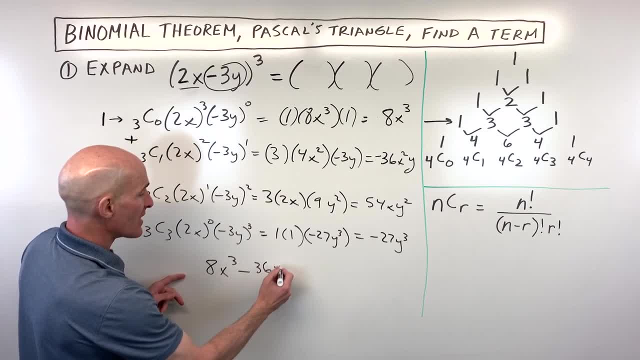 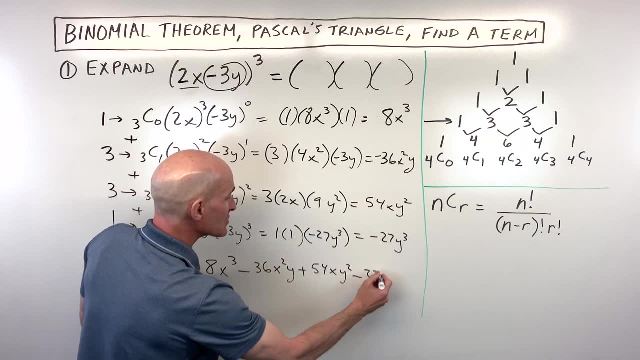 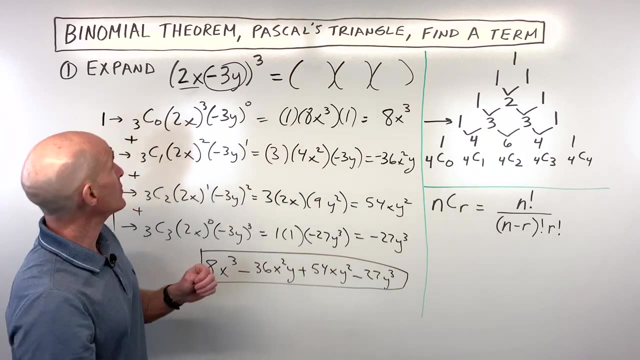 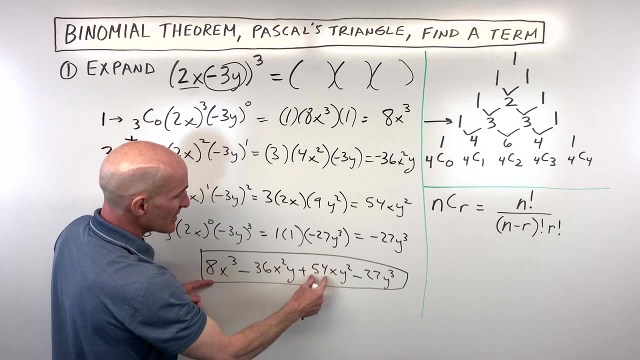 to the third: minus 36x squared y plus 54xy squared minus 27y cubed, and you've expanded it and that's it. Now. one thing to pay attention to is see how this is subtracting. When you're subtracting like this, notice these terms alternate: positive, negative, positive, negative If they were. 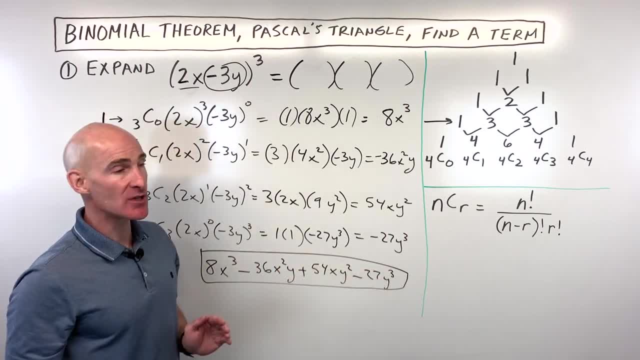 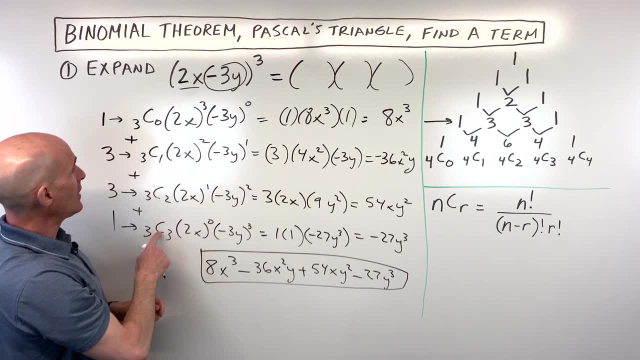 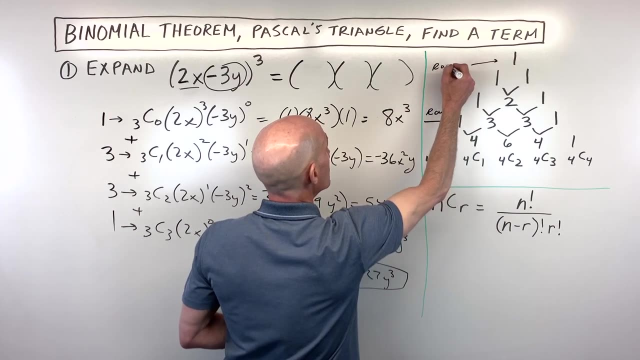 both positive. these would all be positive, all these terms. and the other thing to watch out for here is is that you can use the combinations like I was showing you, okay, or you can just use Pascal's triangle. just go down here to row number three. Again, remember, this starts at row zero. 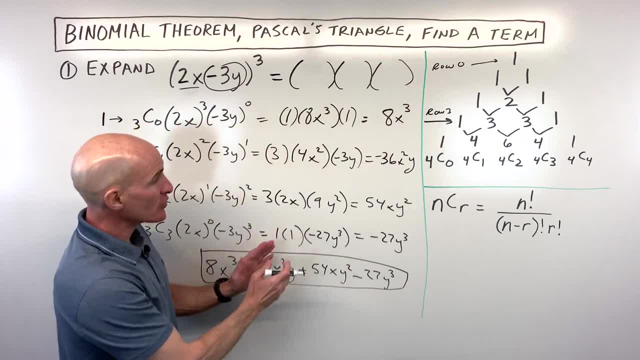 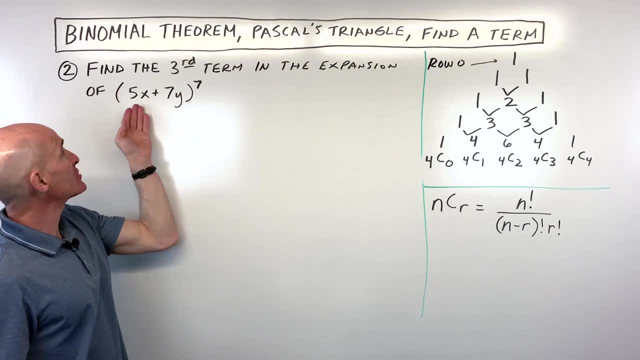 Let's talk about another example where you're just zeroing in on a particular term, not doing the whole expansion. Let's look at that next. So how do we find the third term in the expansion of 5x plus 7y to the? 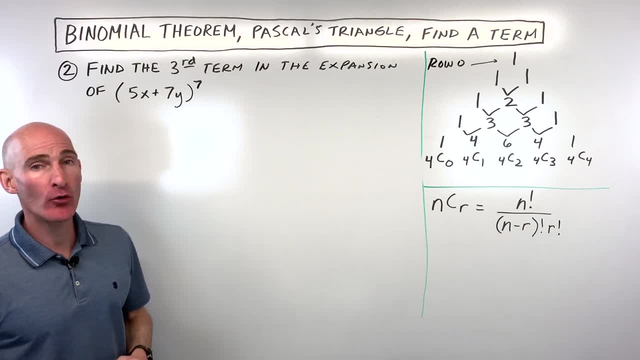 seventh power without having to actually expand the whole binomial using that binomial theorem. Well, what we can do is we can use that pattern we were talking about earlier in the first question. We could say: well, hmm, if I want to go down to the seventh row in Pascal's triangle, right? 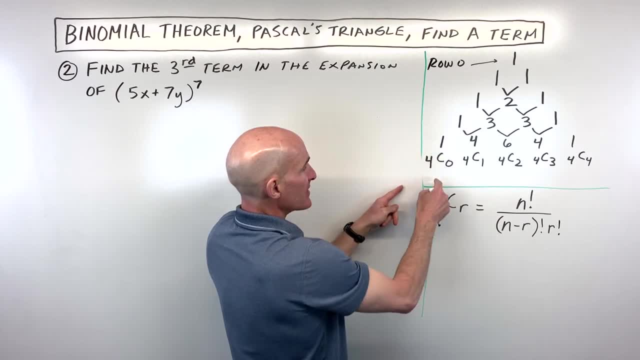 it would start off with 1, and then 7, and then etc. right, but where are those numbers coming from? It would start off with 7 choose 0,, 7 choose 1,, 7 choose 2, etc. So the third term here is actually. 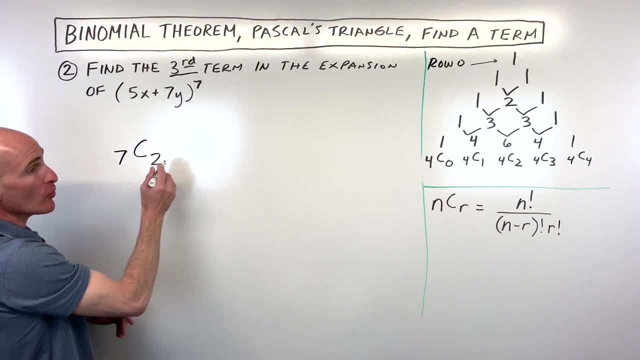 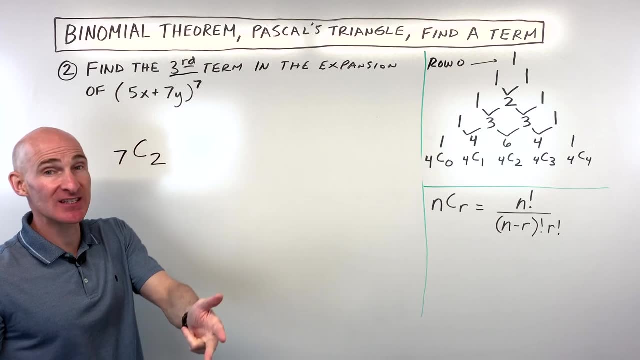 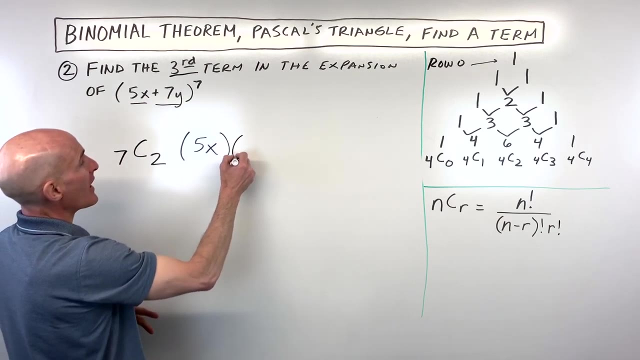 going to be 7c2.. Why 2?? Because we're starting each row with 0.. So this is going to be 7c0, 7c1, 7c2.. That's actually our third term. and then look at this pattern. here we've got our two terms, 5x and 7y. 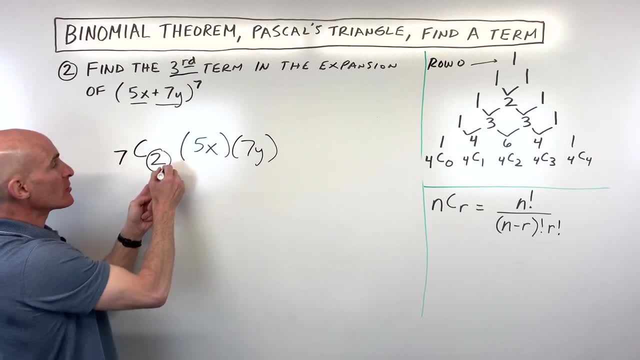 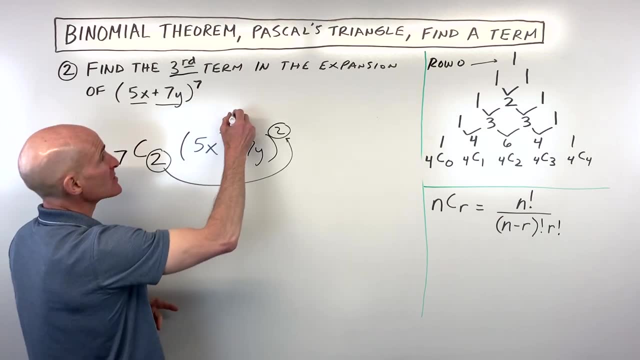 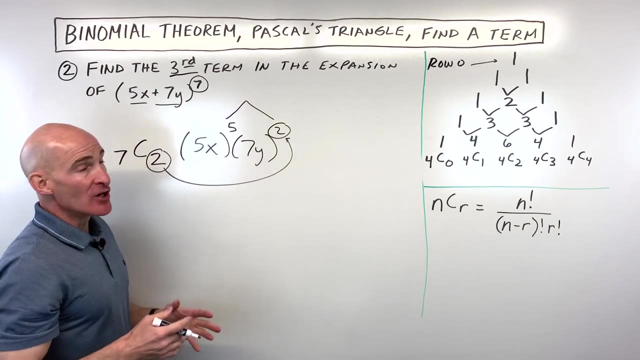 but remember how we said that this r value here and the exponent on the second term. they're always in lock step, they always match. and remember the pattern where we said these two exponents here are going to add up to this power, here the 7. so in this case this has to be to the fifth power. So now we've zeroed in on that. 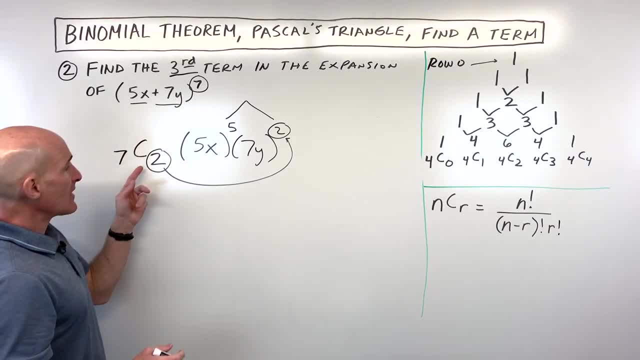 particular term. all we have to do is simplify. So 7c2. you could do this on your calculator if you have a combination key on your calculator, or you can use the factorials, this formula here. So I'll show you if you expand this. the. 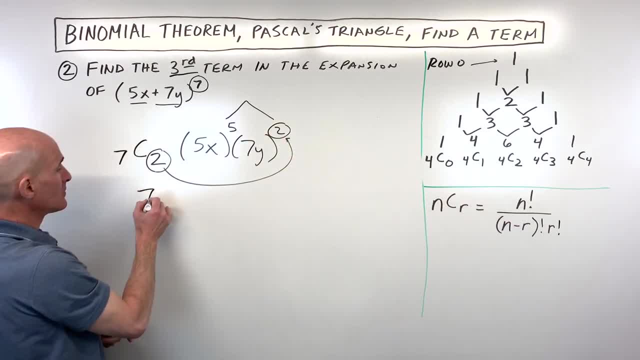 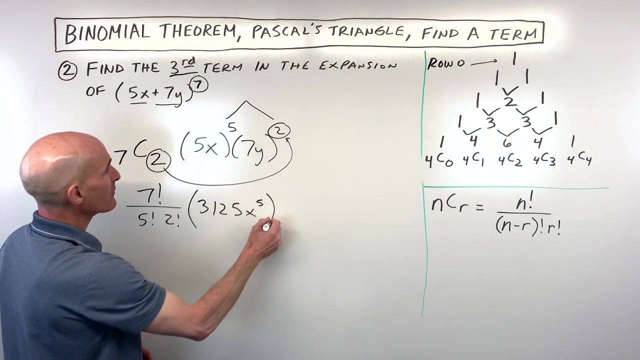 come out to 7 factorial over n minus r, so that's going to be 7 minus 2, which is 5 factorial, and then r factorial, which is going to be 2 factorial. Okay, then we're going to say: well, 5 to the fifth, which is 3125, x to the fifth, 7 squared, that's 49 y squared. Okay, so, 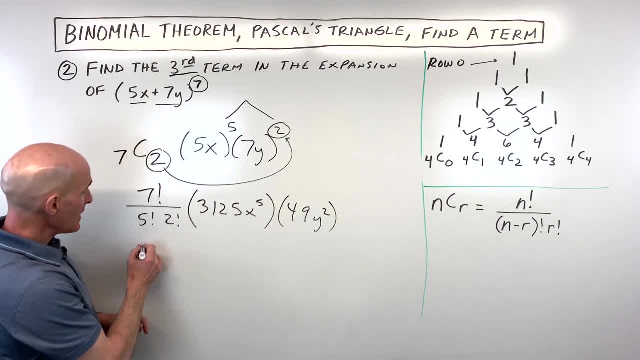 continuing to simplify down here now: 7 factorial represents 7 times 6 times, 5 times, 4 times, 3 times, 2 times 1.. Remember the factorial tells you: start at this number, you multiply down to 1.. Same thing with 5 factorial, that's 5 times 4 times 3 times, 2 times 1 and 2 factorial is 2 times 1.. 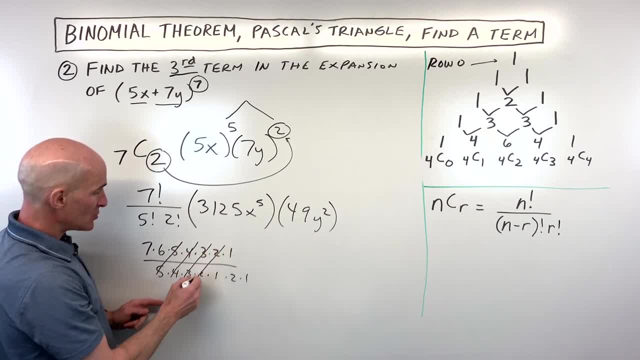 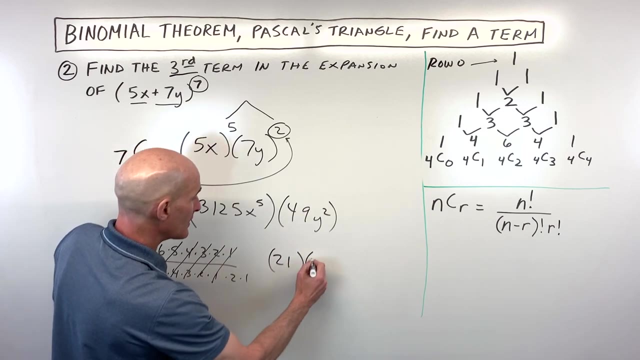 So notice the 5,, 4,, 3,, 2, and 1. cancel numerator and denominator. 7 times 6 is 42. 2 times 1 is 2.. 42 divided by 2 is 21.. So we have, 21 times this whole quantity, 3125 x to the fifth. 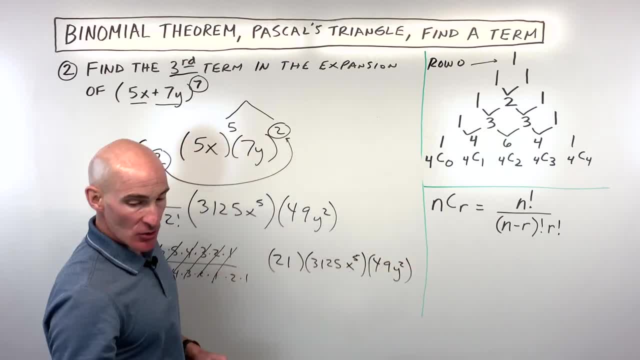 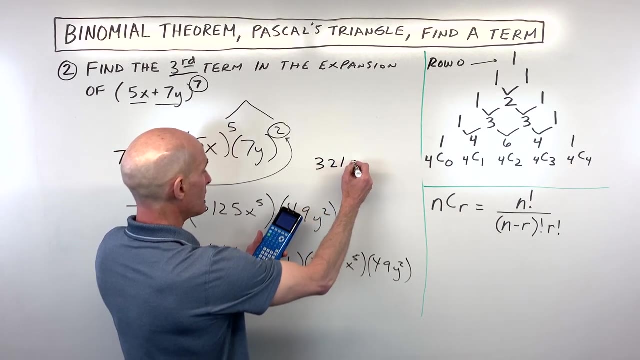 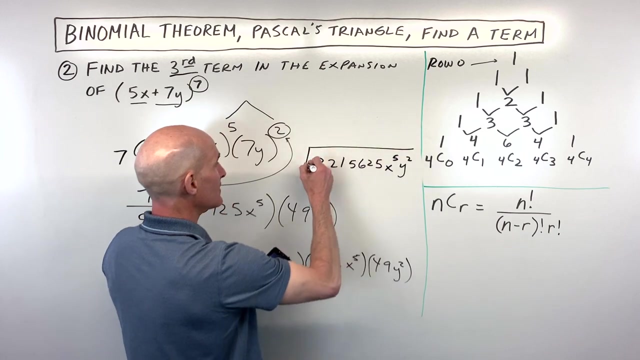 times 49, y to the second. Let's go to the calculator and finish simplifying that That's 21 times 3125 times 49. This is coming out to a large number here. This is coming out to 3, 1, 5, 6, 2, 5, x to the fifth, y to the second, and you've zeroed in in that particular term. Now. 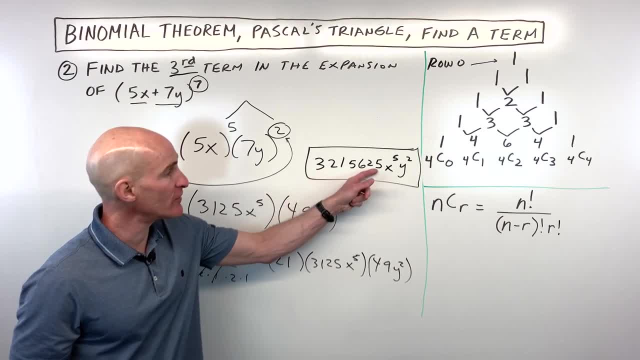 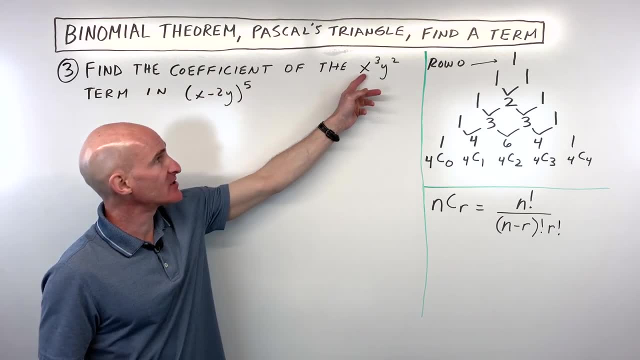 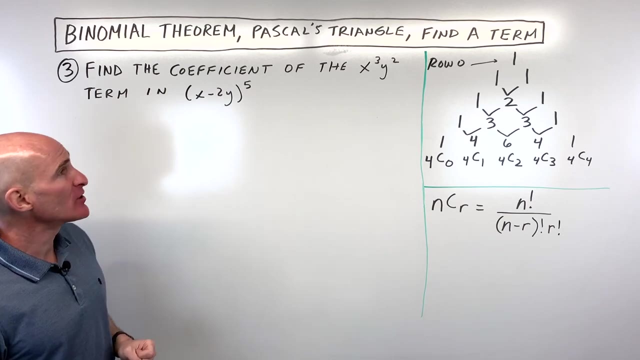 let's talk about a problem that involves just solving for this coefficient in front of the variables. Let's do that in example three. Find the coefficient of the x cubed y squared term in the expansion of x minus 2y to the fifth power. So how do we do that? Well, 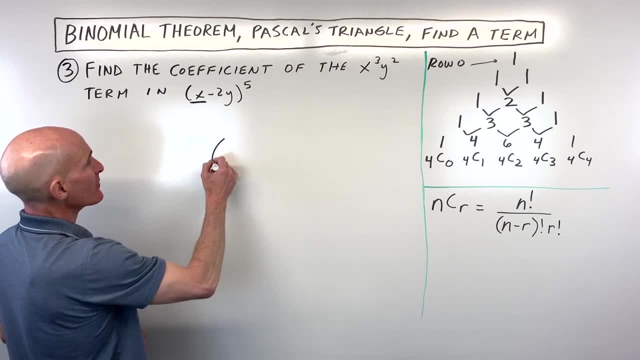 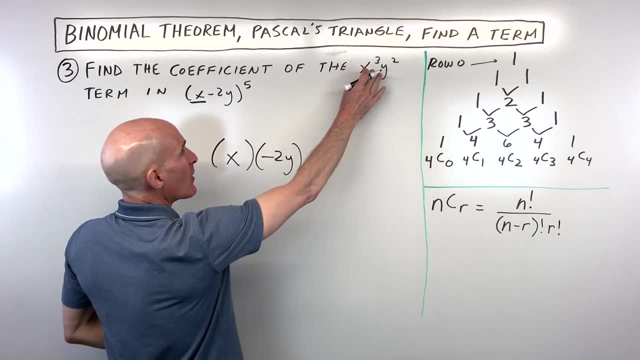 what I like to do is I like to write down my two terms. This is my first term, x. This is my second term, negative 2y, and I know the exponents here because I know I want to end up with x cubed y. 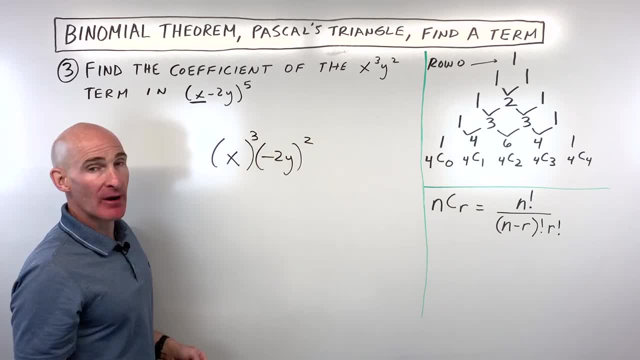 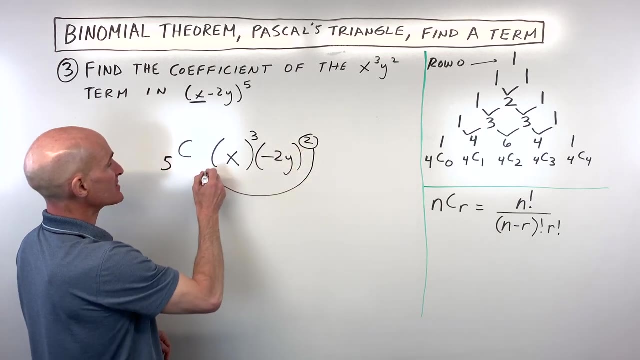 squared. So this has to be to the third power, This has to be to the second power, But we're on the fifth row of Pascal's triangle, right? So this is, uh, to the fifth power. So this is going to be 5 c, and remember the connection here between this second term's exponent and this. 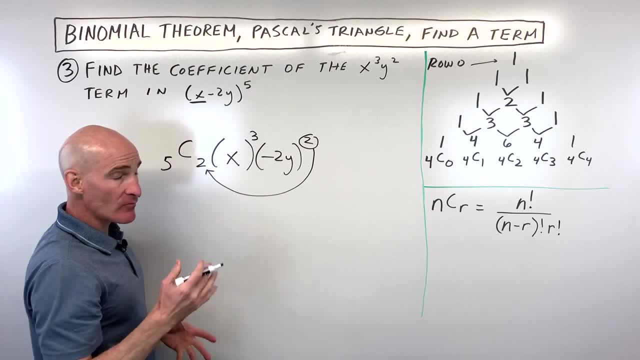 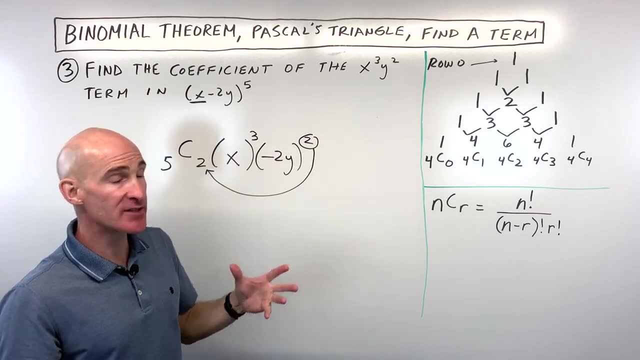 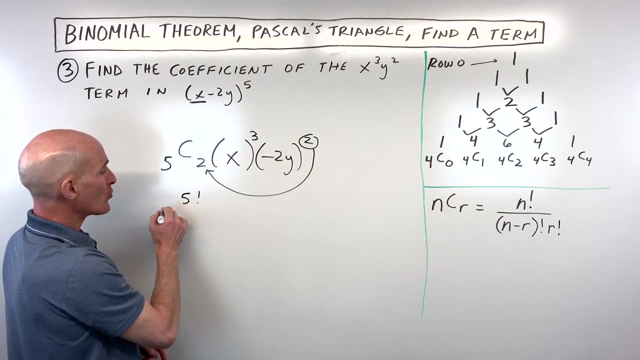 r value. So this has to be 5 c 2.. So now we've zeroed in on the term, but we want to find out just the coefficient, the number that comes in front of this, x cubed, y squared. So let's simplify a little bit more. So 5 c 2, using our combination formula, is going to be 5 factorial. 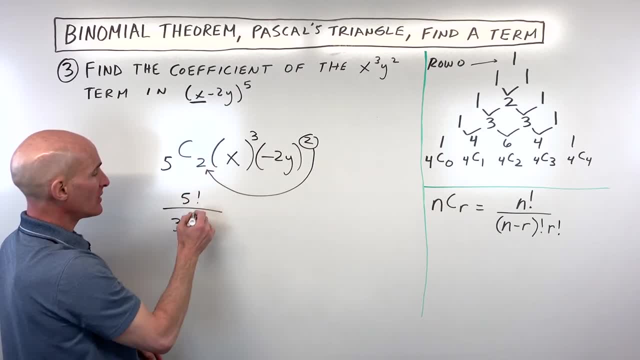 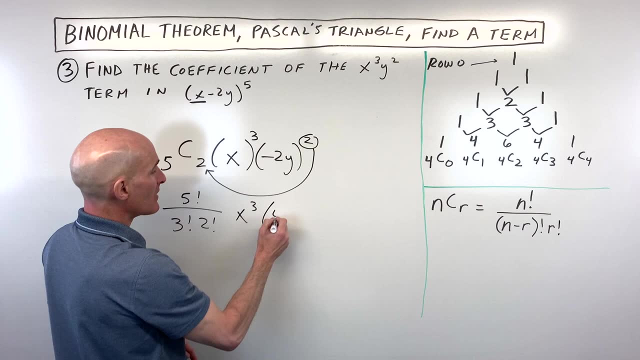 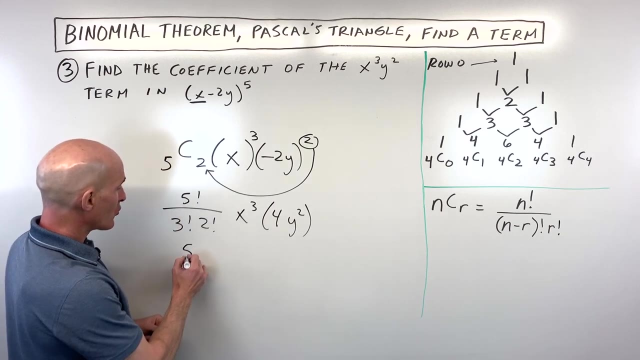 over 5 minus 2: 3 factorial times. 2 factorial. This is going to come out to x cubed and negative. 2 squared is going to come out to 4.. y squared- a negative times a negative is a positive 4.. Now, if we simplify here: 5 factorial. 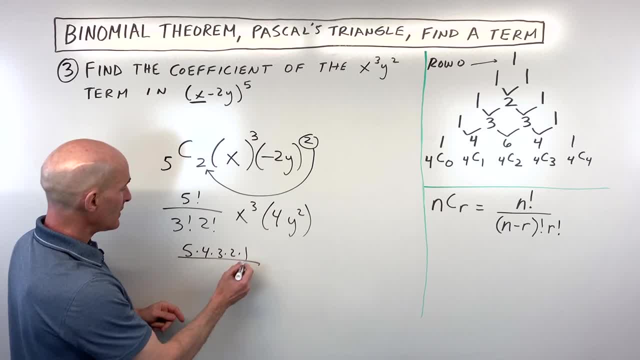 is 5 times 4 times 3 times 2 times 1.. 3 factorial is 3 times 2 times 1 and 2 factorial is 2 times 1.. So you can see that 2, the 1 are canceling numerator and denominator. These 3's are: 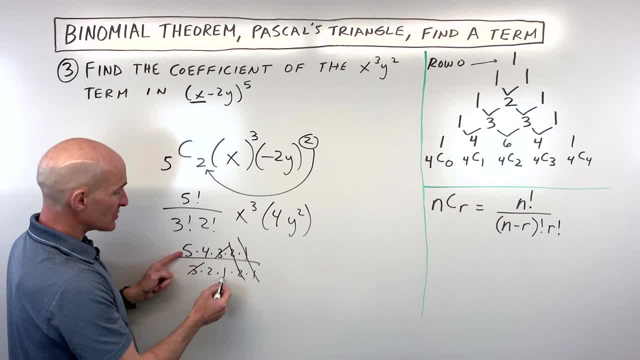 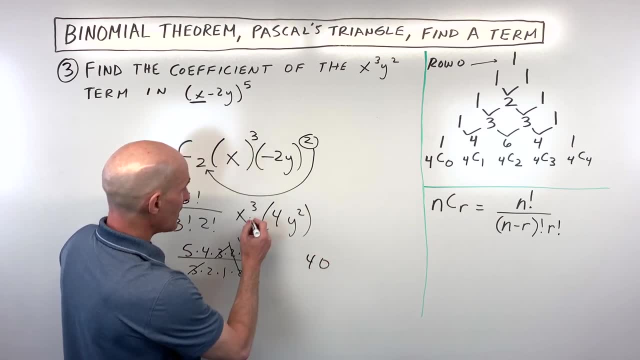 canceling This comes out to 20.. This comes out to 2.. 20 divided by 2 is 10.. So we have 10 times 4, which is 40 x cubed y squared. We just want the coefficient, So we're just after this number that. 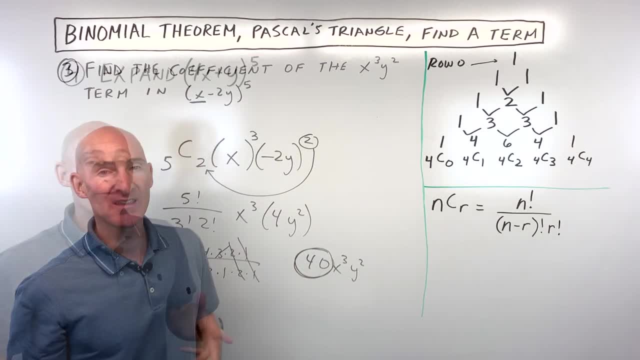 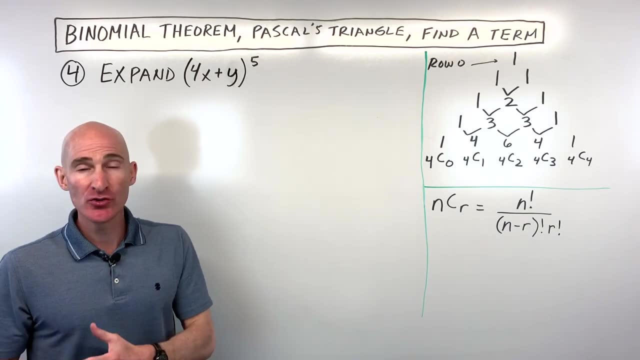 comes in front here. So your final answer would be 40.. Okay, for example, number 4, 5 and 6: they're going to basically be repeats of example 1, 2 and 3.. So see if you can do these problems on your own. 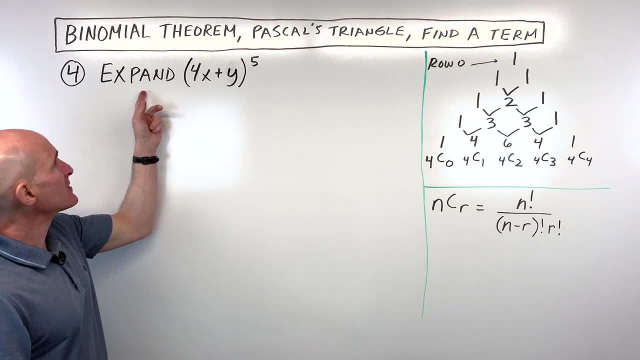 We'll go through them together. and let's dive into number 4. now. It says: expand 4x plus y to the 5th power. Well, if I was going to do this, I would use either the combinations or I would go down to the 5th row in Pascal's triangle. So here, 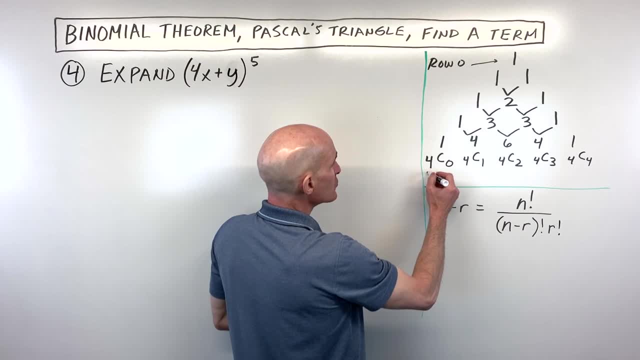 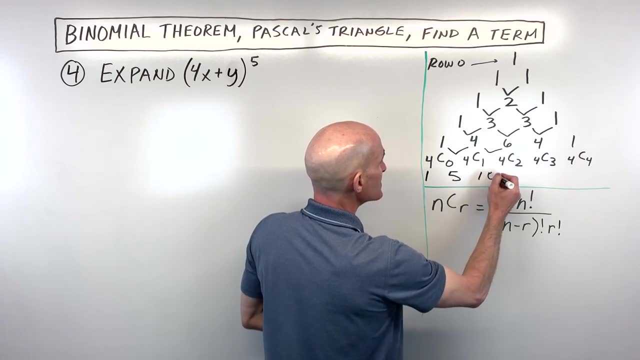 previously I went down just to the 4th row, So remember each row starts with 1.. Then I add the two numbers above it. So 1 plus 4 is 5.. 4 plus 6 is 10.. 6 plus 4 is 10. again, 4 plus 1 is 5 and 1.. 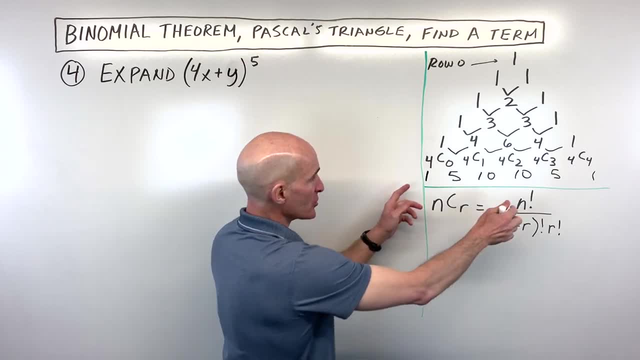 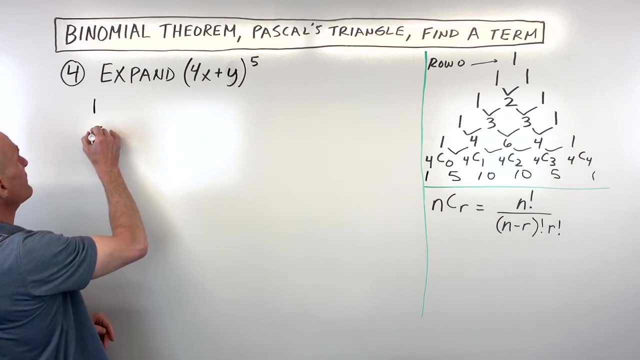 Remember it always begins with 1 and ends with 1.. One thing you'll also notice is it's symmetric, See 1, 5, 10, right, Okay, so we're going to use those coefficients: 1, 5, 10, 10, 5 and 1.. Remember where they come from. They really 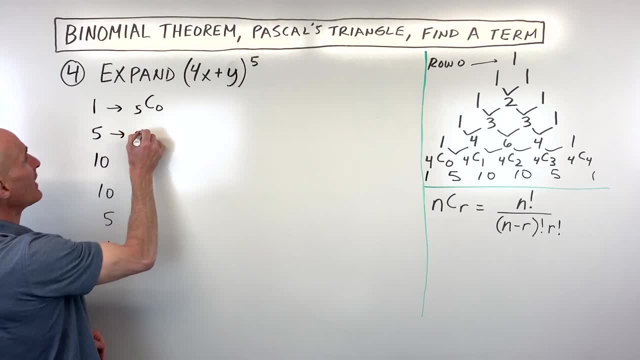 come from the 5c0,, 5c1,, 5c2,, 5c3,, 5c4, and 5c5.. Then we take our first term here, which is 4x, and we take that to the 5th power and we go in descending orders. 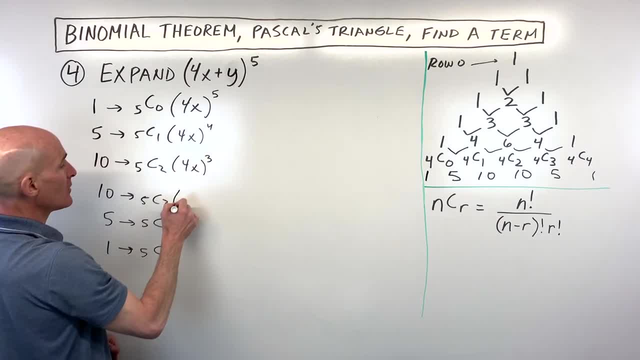 4x to the 4th, 4x to the 3rd, 4x to the 2nd power, 4x to the 1st power and 4x to the 0th power. Then we take the second term, which is positive y, or we could just say y. We start at the 0th power. 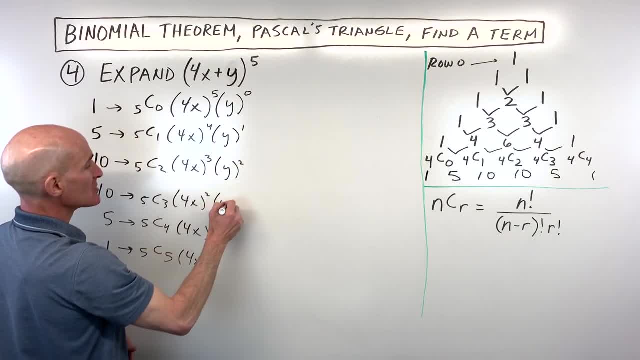 and we go in ascending order, meaning we're going up. So y squared, y to the 3rd, y to the 4th, y to the 5th, And notice these are all multiplied together and then each individual term is added to the next term, So there's like a plus sign in between each of these terms. So now let's. 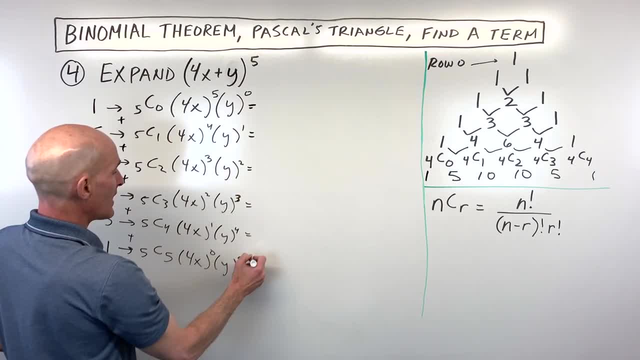 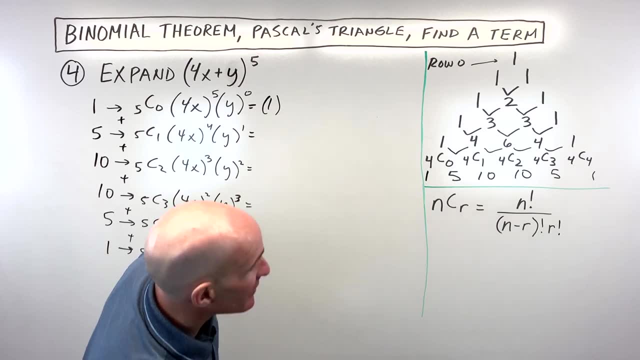 go ahead and simplify this down a little bit. And so what do we get? It looks like we're getting 5c0, which is 1. 4 to the 5th power. I'm going to have to go to the calculator on that one: It's 1024.. 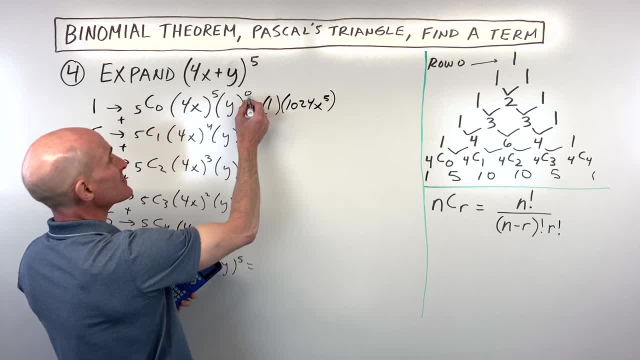 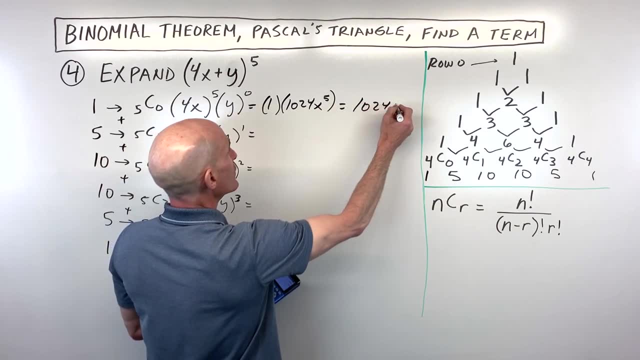 x to the 5th And then y to the 0. Anything to the 0 power is 1.. So 1 times 1 is 1.. So this is just coming out to 1024 x to the 5th. That's our first. 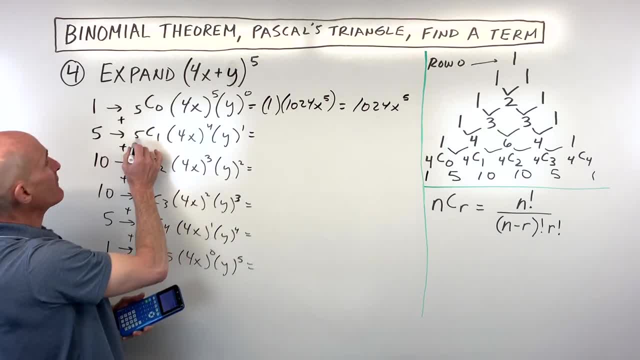 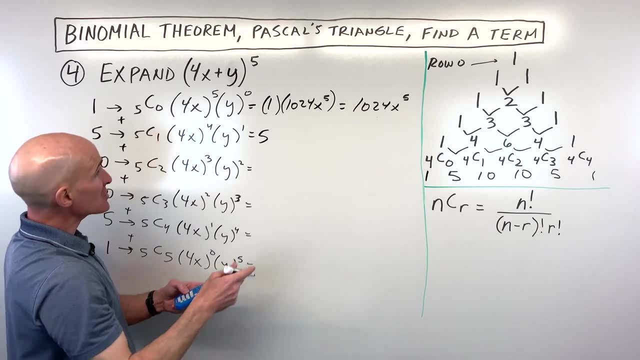 term in this expansion, Second term, we've got 5c1, which is 5.. And then we've got 4 to the 4th power, which is 256.. x to the 4th, y to the 1st. 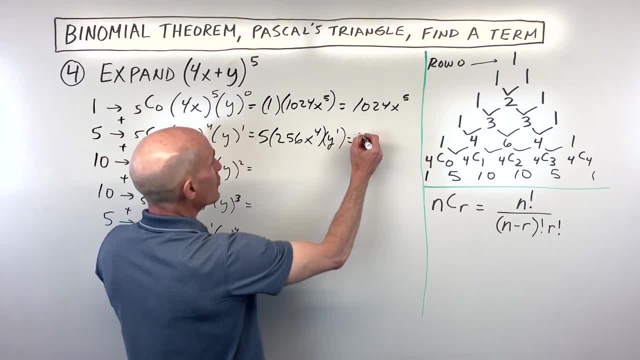 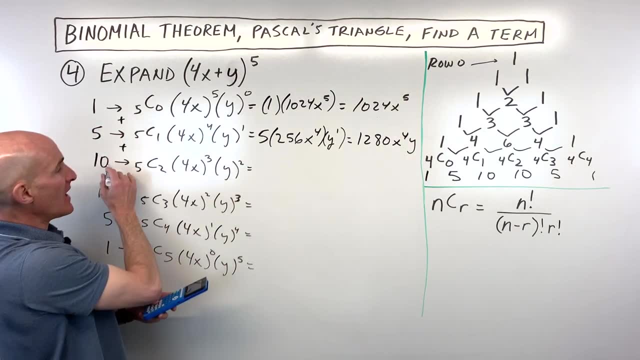 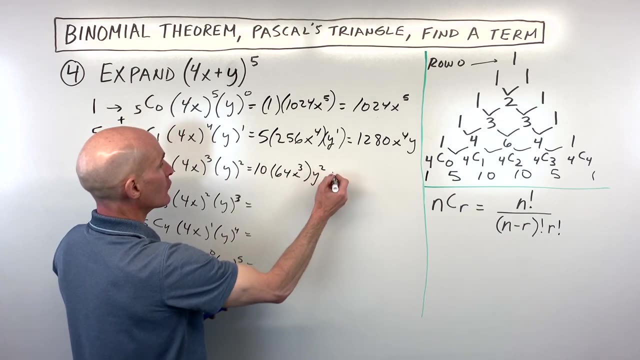 Okay. so if we multiply that together that comes out to 1280. x to the 4th, y, 5 c2, that's 10.. So we have 10.. 4 cubed is 64, x cubed And y squared. So if we multiply that together we get 640. 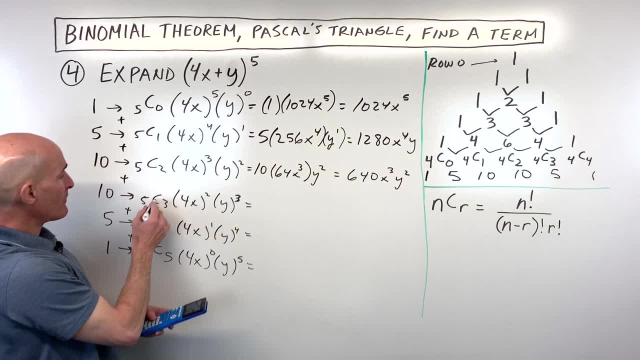 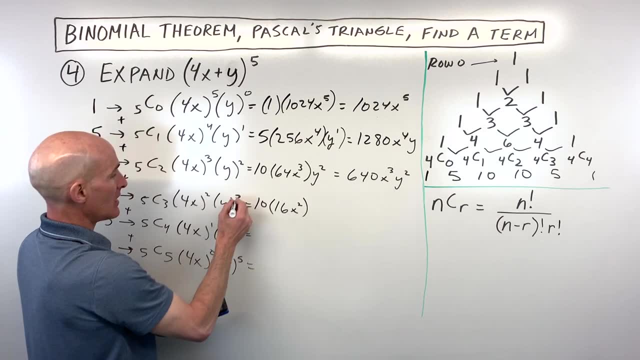 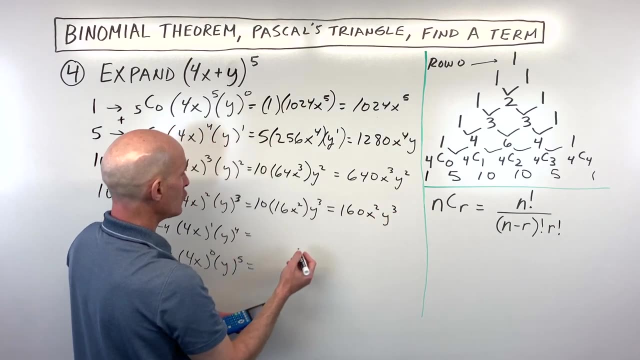 x cubed, y squared. And then for the next term, 5c3 is 10.. So we have 10.. 4 squared is 16, x squared. So if we multiply that together you can see we're getting 160x squared- y cubed. 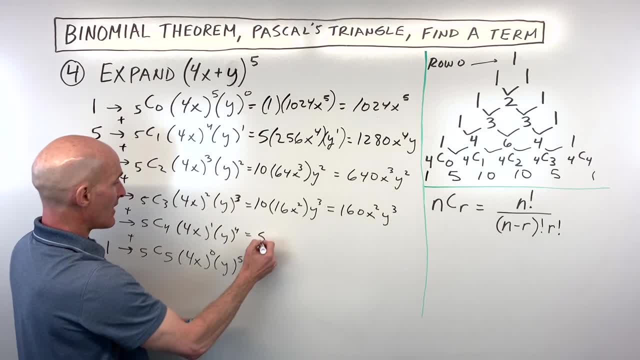 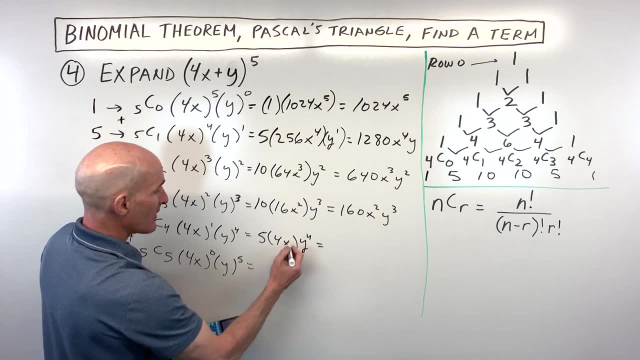 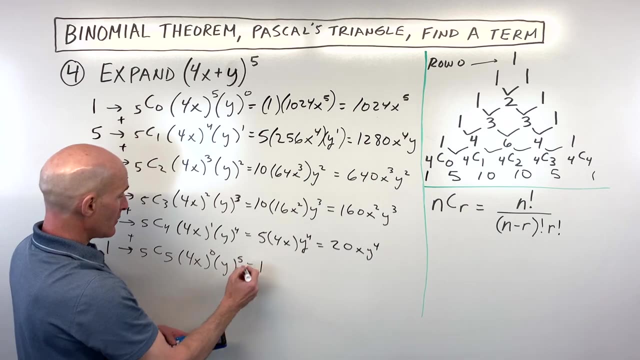 This term, 5c4 is 5, so we have 5 times 4x to the first is 4x, y to the fourth, And if we multiply that together we're getting 20xy to the fourth. And the last one, 5c5, is 1,. 4x to the zero is 1, y to the fifth. 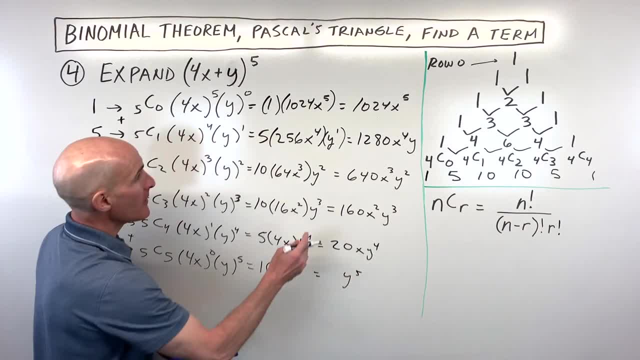 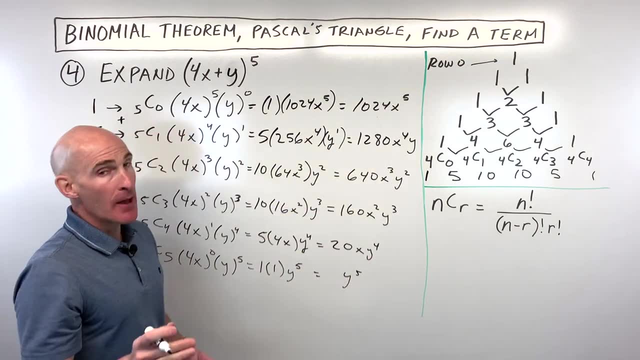 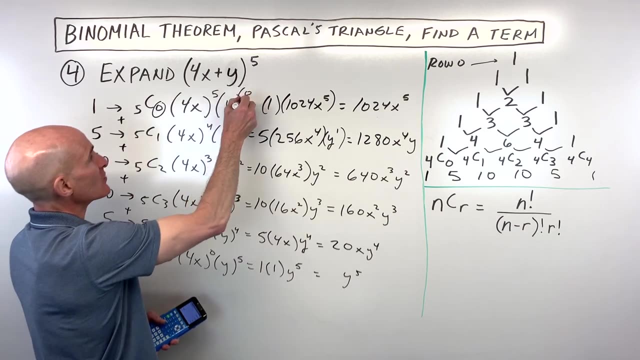 So that just simplifies. to y, to the fifth, And then all these terms are added together. Now you can write it horizontally. I have it here vertically. Normally we write it horizontally, But again, notice some of the patterns here. See how this first term we had 5c0, and this r value is matching with this second term's power. 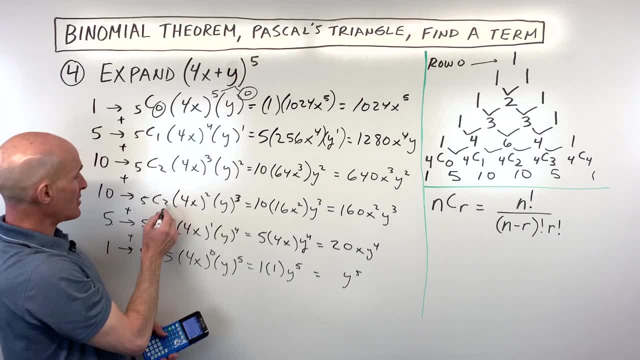 We also notice that 5 plus 0 is 5.. Or if I jump down here see how this is like: r value is 3, and the second term's power is 3.. They match. 2 plus 3 is. 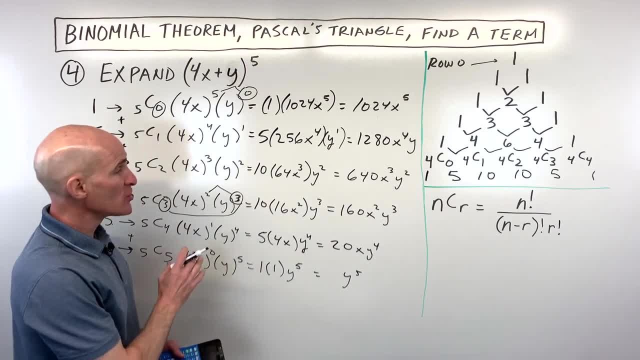 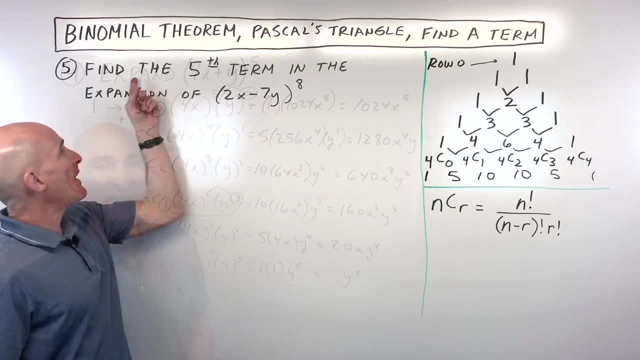 5. See that exponent that power. So we're going to use that in the next problem where we zero in on just a particular term without having to do the entire binomial expansion. Find the fifth term in the expansion of 2x minus 7y to the eighth power. 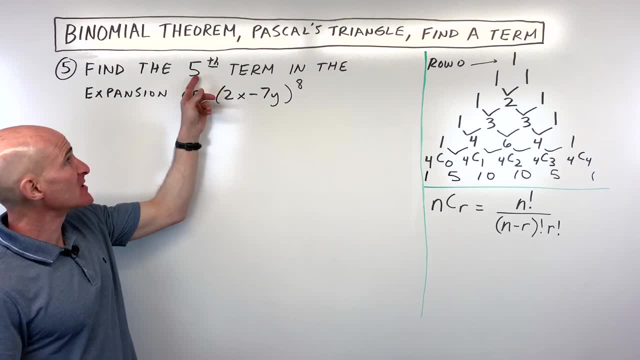 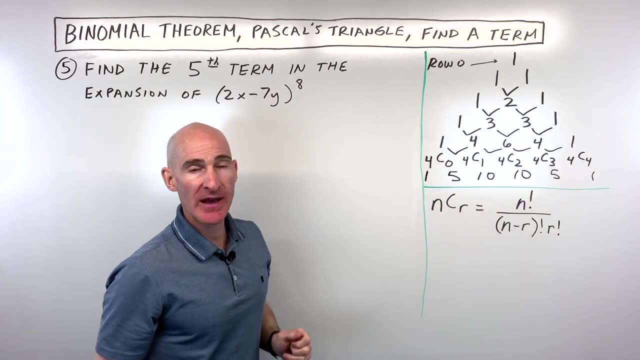 So we don't want to take the time to do the entire expansion, We just want to zero in on this fifth term. But notice, this is to the eighth power. So what we could do is we could go down to the eighth row of Pascal's triangle, keep expanding. 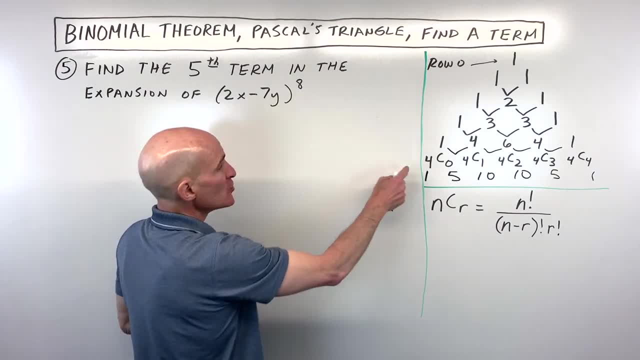 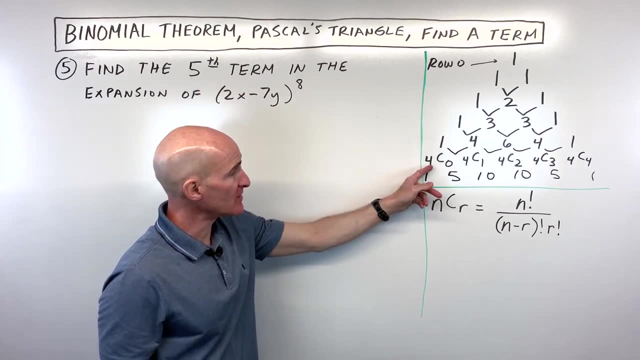 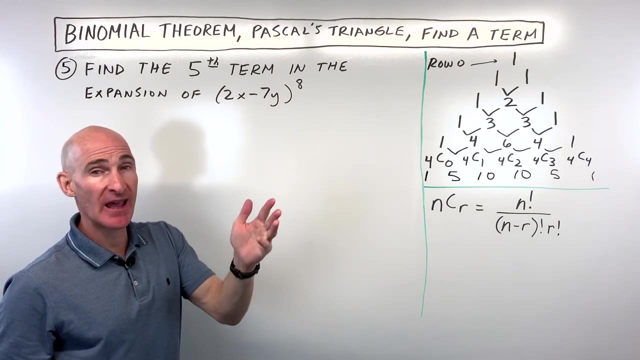 That would take a little bit of time. The other way to do it is we could use the combinations to help us to write that eighth row And if we want the fifth term, knowing that this always starts with 0, that's going to be 8c0, 8c1,, 8c2, 8c3, 8c4 is actually going to be for our fifth term. 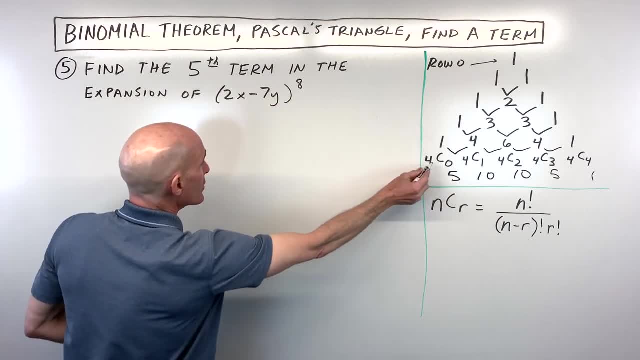 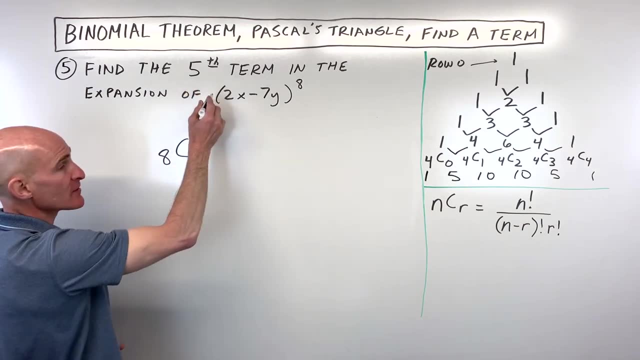 Notice. it's one less because we're starting at 0 right here, So this is going to be 8.. That's coming from this power. That's the row we go to C4.. One less than the fifth term because we're starting at 0.. 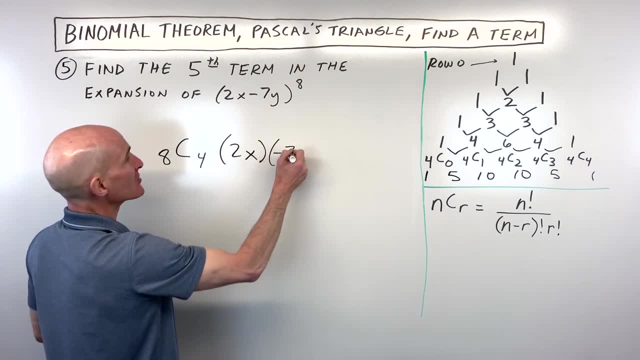 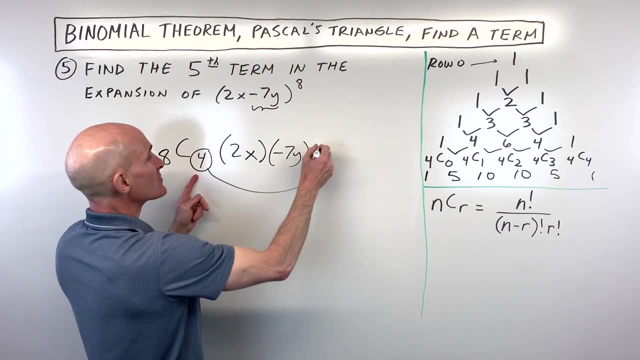 Then we're going to take our first term, which is 2x, Our second term, which is negative, 7y, And remember the pattern here: This r value and the second term's exponent they match, They're the same. 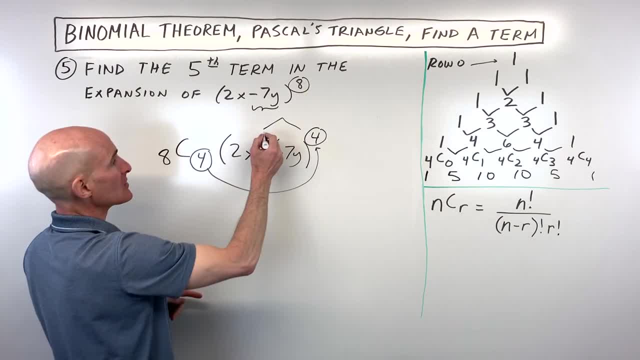 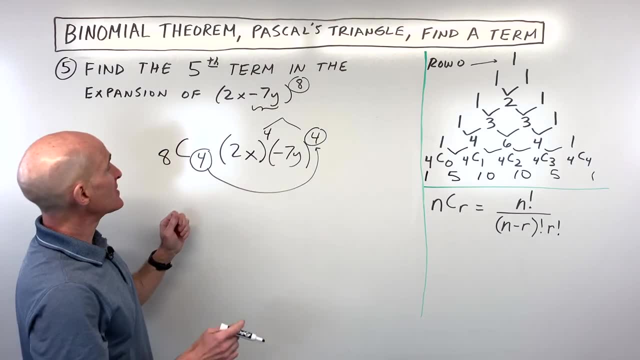 These two exponents have to add up to this power here, 8.. So that means that this has to be to the fourth power, because 4 plus 4 is 8.. So now we've zeroed on that particular term, Let's just go ahead and simplify. 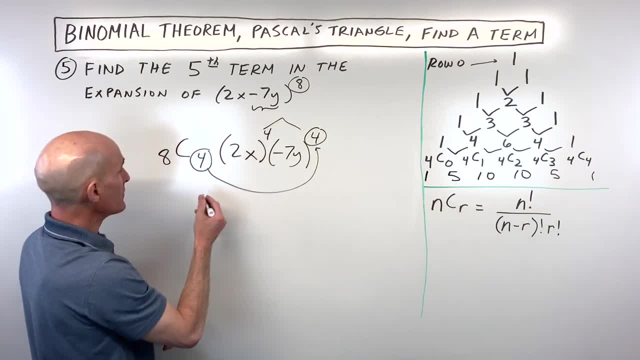 So 8c4.. Using our combinations formula, here it's going to be 8 factorial over 8 minus 4, 4 factorial, 4 factorial. Okay, 2 to the fourth we know is 16.. x to the fourth. 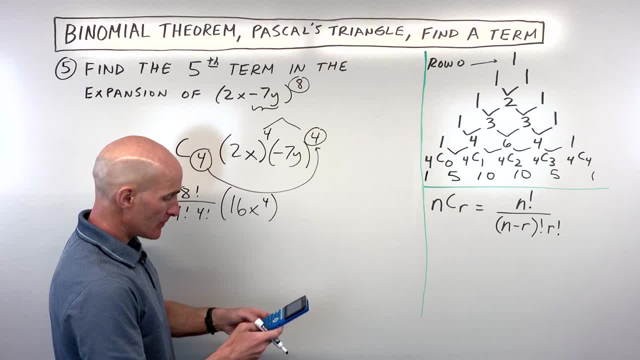 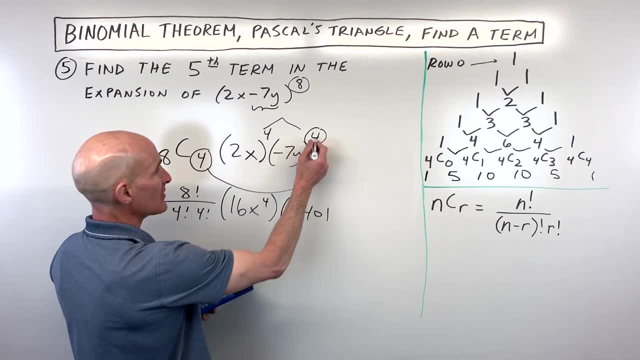 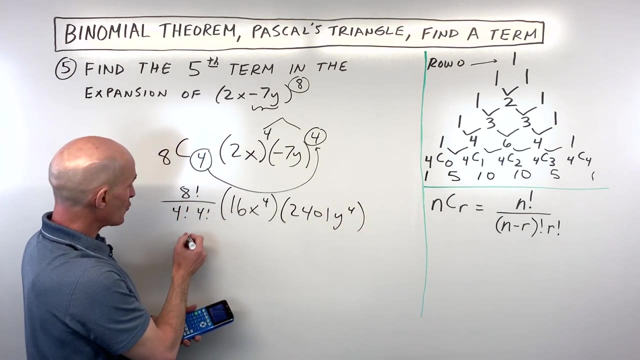 And negative 7 to the fourth. Let's do that on the calculator. That's coming out to 2,401 positive, because a negative times, a negative times, a negative is an even number of times. And so now let's simplify this. So 8 factorial is really 8 multiplied all the way down to 1.. 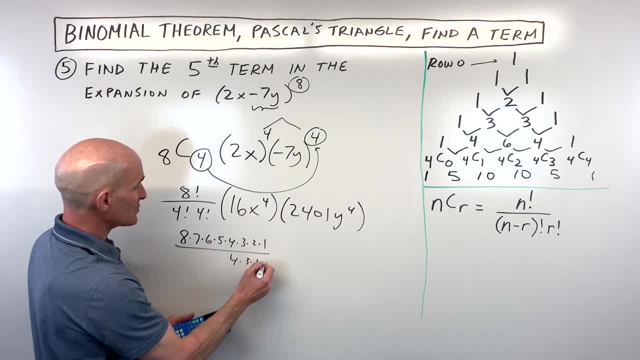 4 factorial is 4 times 3 times 2 times 1.. And this 4 factorial 4 times 3 times 2 times 1.. You can see these are canceling numerator and denominator. Let's see: 4 times 2 is 8.. 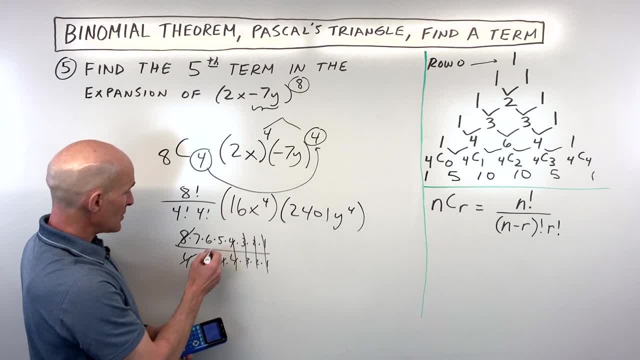 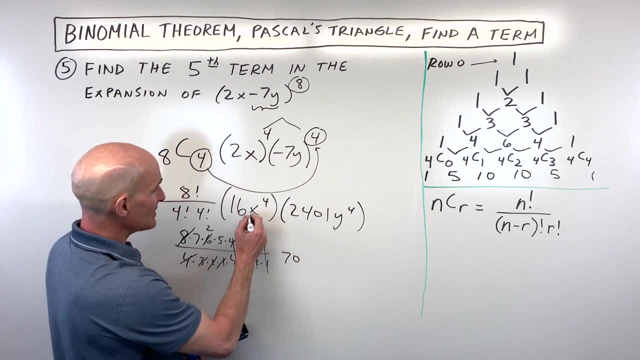 That cancels with this 8.. 3 times 1 is 3.. That goes into 6 twice 2 times 5.. 5 is 10.. Times 7 is 70. So what we have is 70 times all of this. 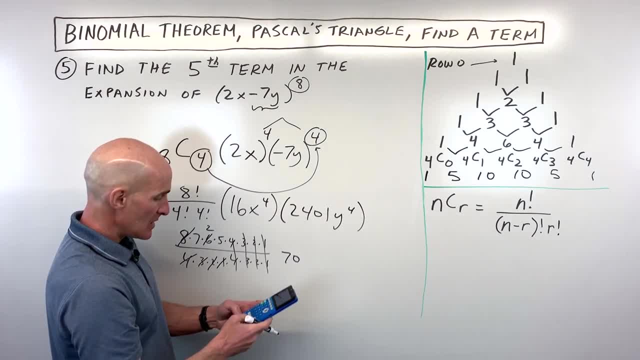 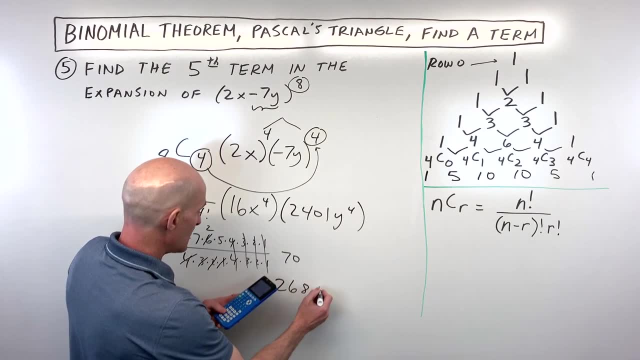 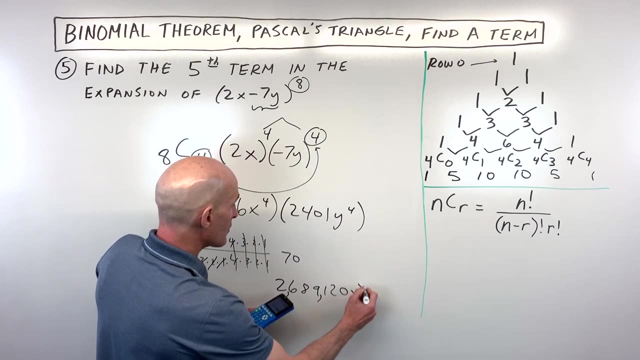 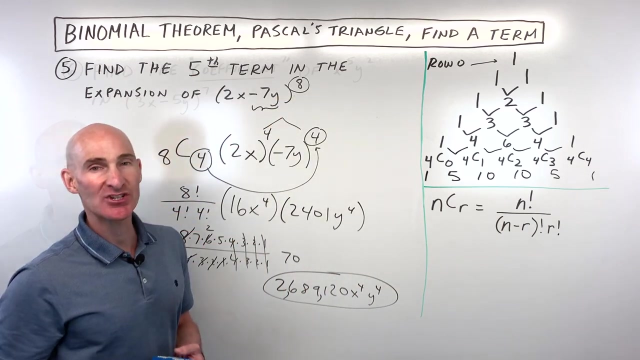 So let's go ahead and do that on the calculator: 70 times 16 times 2,401 is giving us 2,689120. x to the fourth, y to the fourth, And that's just that particular term, the fifth term in this binomial expansion. 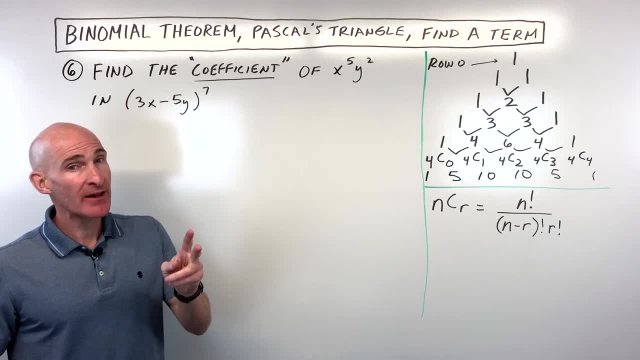 Okay, Before we jump into this next problem, which I'm going to actually have, another problem after this as well, a bonus problem. So we'll actually have seven problems in this video, And congratulations for sticking with me this far. You must be pretty dedicated. 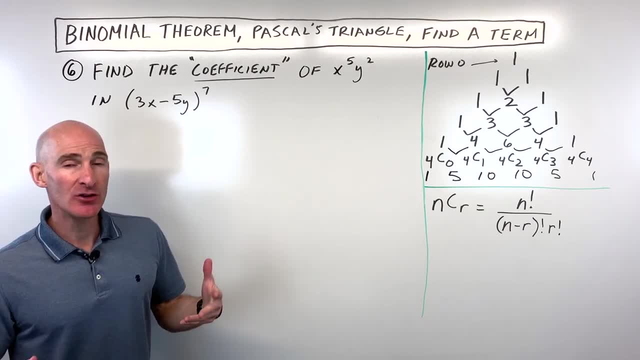 I just wanted to let you know if you like the way that I'm explaining things and you would like to learn more about either Algebra 1 or Algebra 2, College Algebra. I have video courses for sale with links in the description below. 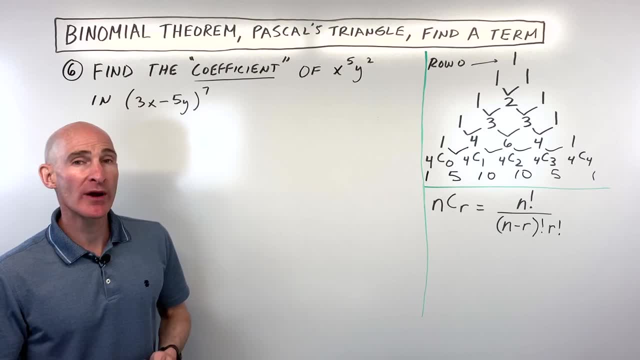 So check out those video courses if you want to learn more about Algebra 1,, Algebra 2, College Algebra, And if you just want to support me, I'm going to be happy to help you out. I'll see you next time. 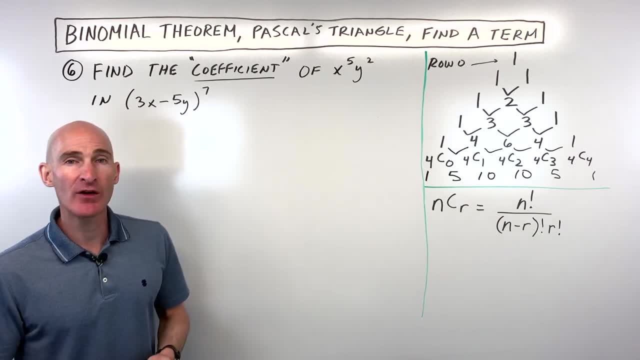 Bye. If you want to support the channel, consider joining as a channel member. for a few dollars a month, You can help support the content that I'm putting up here for you guys, And I'd really appreciate it. So thank you for that. 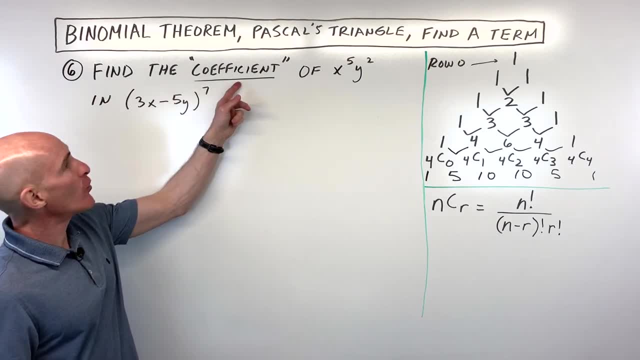 But let's jump into number six. So can you do this problem? Can you find the coefficient, meaning the number that comes in front of this variable expression, x to the fifth, y to the second, in the expansion of 3x minus 5y to the seventh? 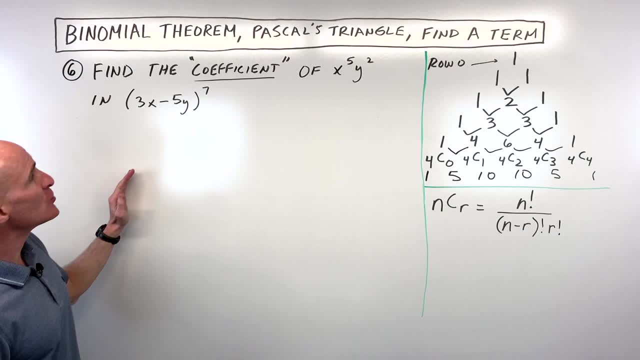 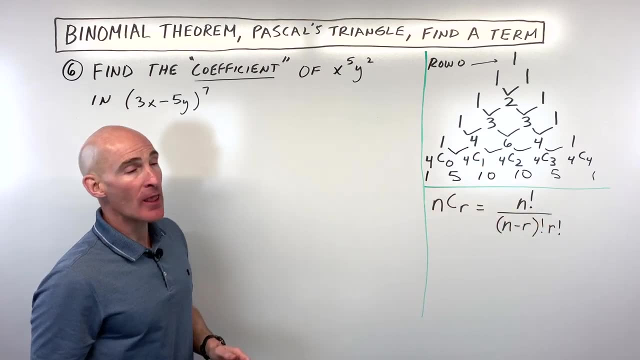 How would you do that one? Well, go ahead and pause the video, See if you can do it, And in the meantime, what I would do is I would either go to the next one, which is go down to the seventh row in Pascal's triangle- if I had that written out- or I can use the. 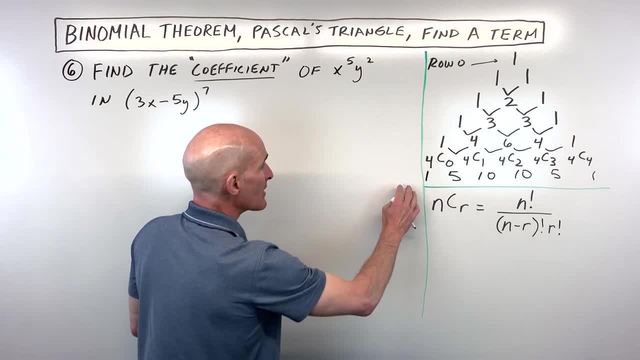 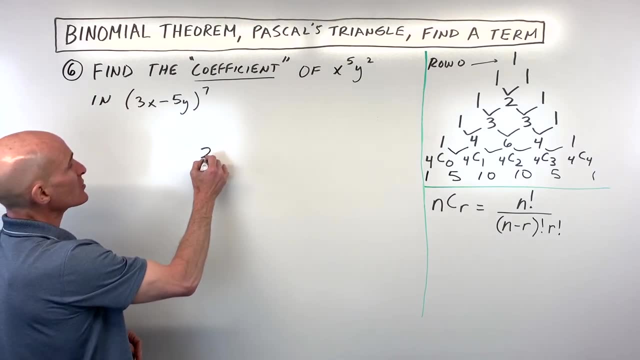 pattern of the combination. So it would start off with 7c0,, 7c1,, et cetera. right, And I know that I'm dealing with these two terms here, which are 3x and negative 5y. 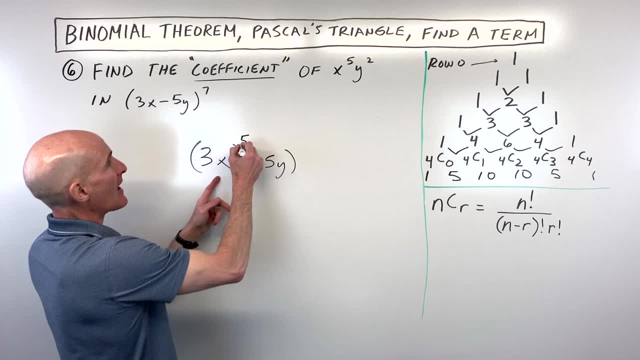 okay, And I know that these exponents have to be 5, because I want to end up with x to the fifth, and this has to be 2.. And this makes sense, because 5 plus 2 adds up to this exponent here, 7.. 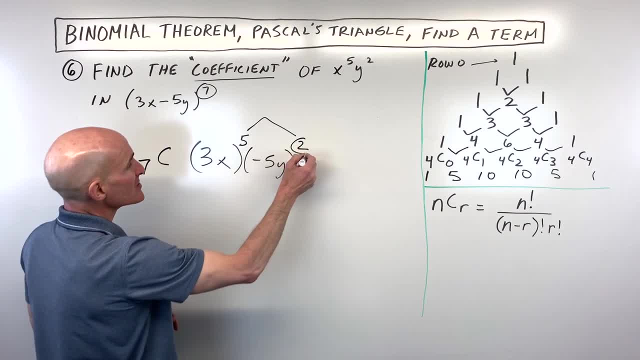 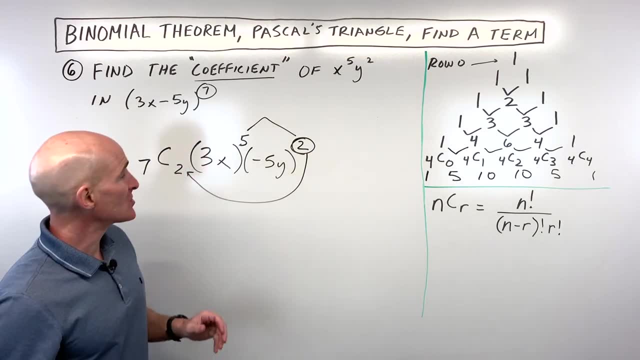 And again we're on the. We're on the seventh row and remember the pattern where this second term's exponent is the same as this r value right here. so that's a match. So now all we have to do is just simplify this. 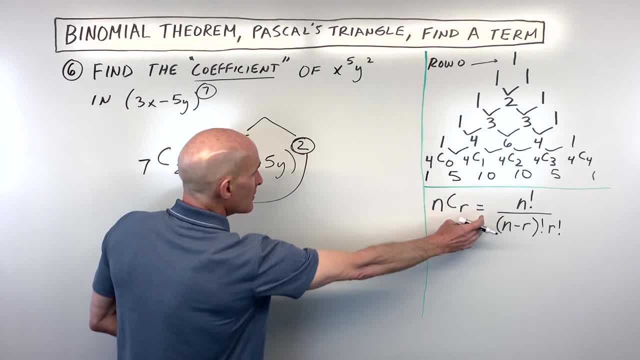 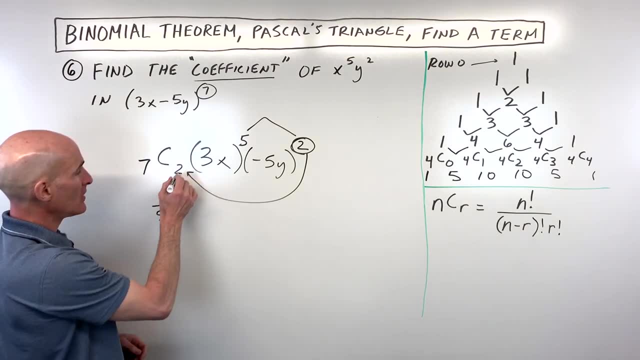 7c2,. you can do this on your calculator or you can use the formula, the NCR formula. That would be 7 factorial over 7 minus 2, 5 factorial 2 factorial 3 to the fifth is 243.. 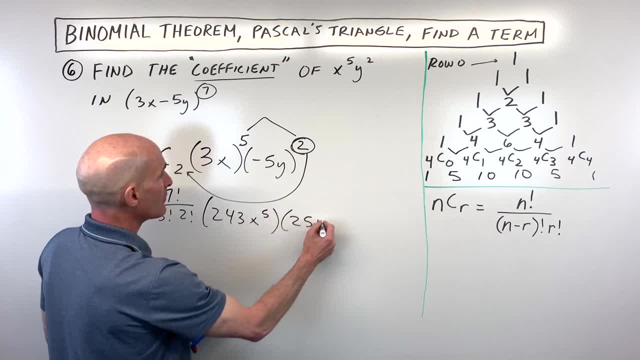 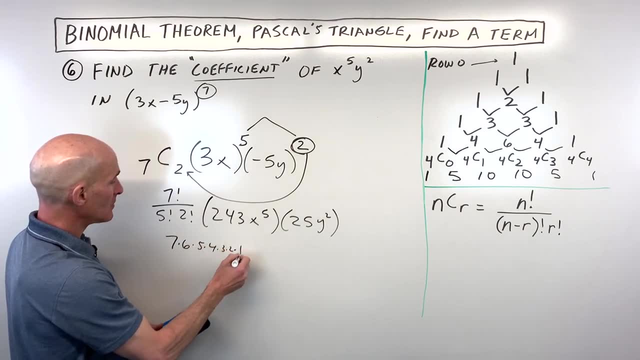 x to the fifth, and negative 5 squared is 25y squared. If we simplify this, 7 factorial is 7 times 6 all the way down to 1.. 5 factorial is 5 all the way down to 1, multiplied together, and 2 factorial is 2 times 1.. 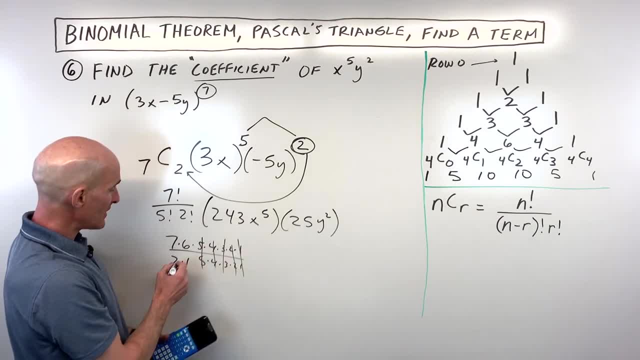 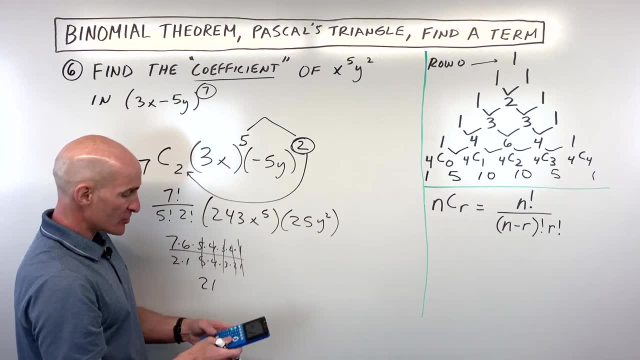 So you can see the 5,, 4,, 3,, 2, 1 cancel numerator and denominator. 42 divided by 2 is 21.. So this would be 21 times these other terms. So this is going to be 21.. 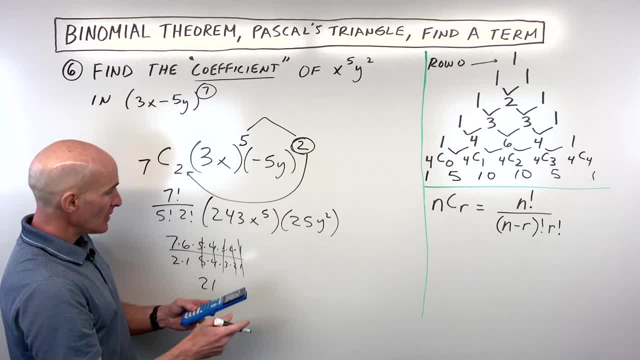 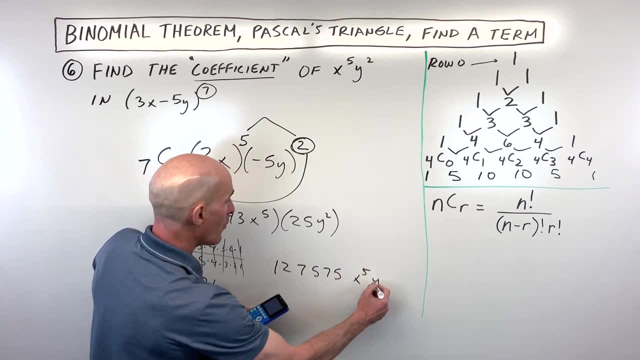 Times 243, times 25,, which comes out to 1, 2,, 7,, 5,, 7, 5, x to the fifth y squared. But we just want the coefficient, That's the number that comes in front of x to the fifth y squared. 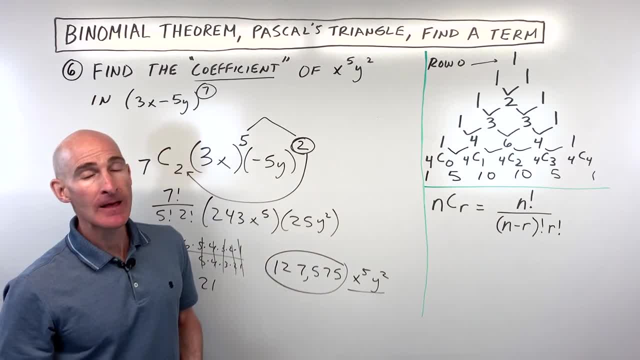 So just the 127,575.. Let's go ahead and take a look at a bonus question here involving imaginary numbers. This is a little bit more challenging. See if you can do this last problem: 2 plus i. 2 plus i to the fourth power. 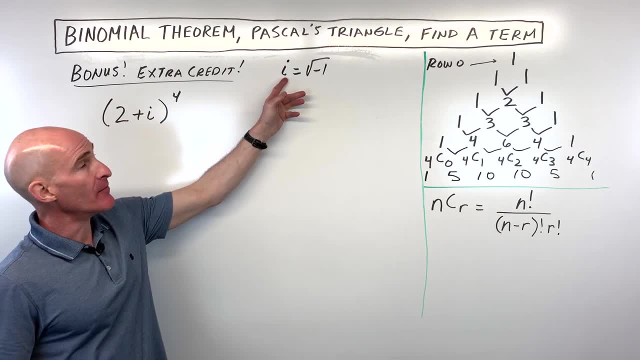 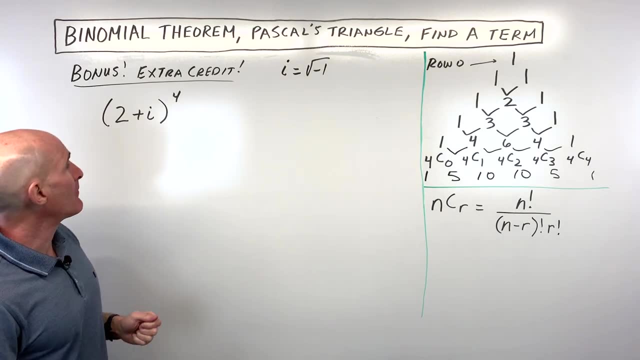 How would you expand that? And the i represents the imaginary i, where it equals the square root of negative 1.. So how would you expand that and simplify it? Write it as a complex number in standard form, a plus bi form. So this is kind of a little bit more challenging, but it's the same idea. 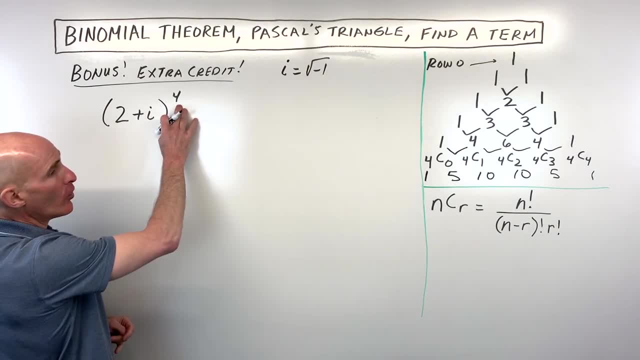 You have a binomial, two terms. We're on the fourth row, right, So this would be 1, 4,, 6, 4, and 1.. Those are our coefficients, So let's write that down, And then we have. 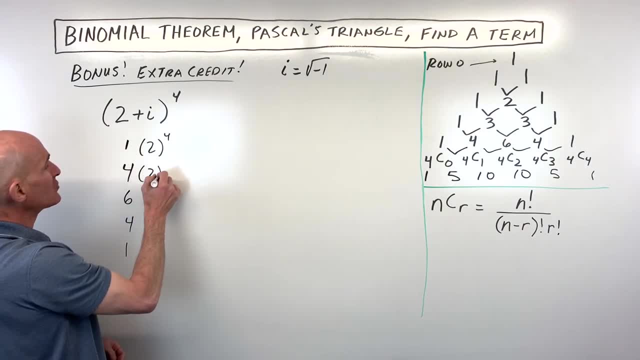 We have 2, our first term- to the fourth power, 2 to the third, 2 to the second. We're going in a descending order: 2 to the first and 2 to the zero. We take our second term, which is i, and we go to the zeroth power and we go in ascending order. 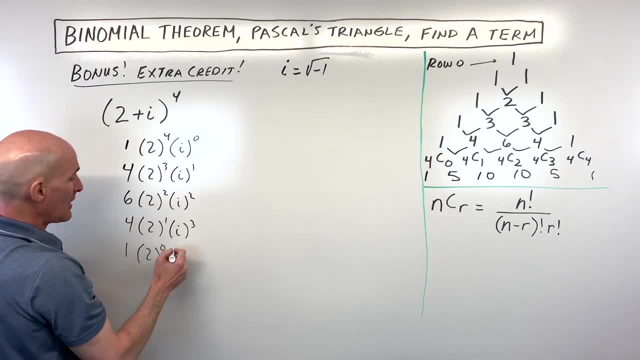 We go up And then all we have to do here is simplify. So 2 to the fourth, we know, is 2 times 2 times 2 times 2.. That's 16.. Times 1 is 16.. Anything to the zero is 1.. 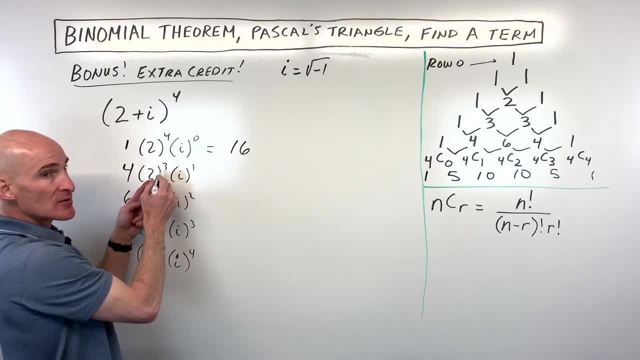 So this comes out to 16.. 2 cubed is 2 times 2 times 2.. That's 8.. Times 4 is 32.. Times i, So that's i, 2 squared is 4.. Times 6 is 24.. 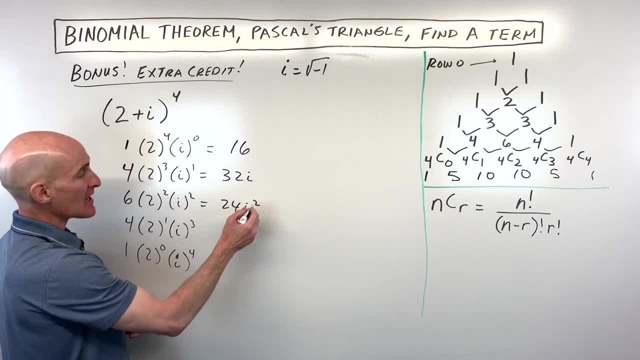 i squared. Okay, now, i squared is how much? Well, i squared is equal to negative 1.. So it's i times i, which is i squared, That's negative 1.. So this would really be equal to negative 24, because negative 1 times 24.. 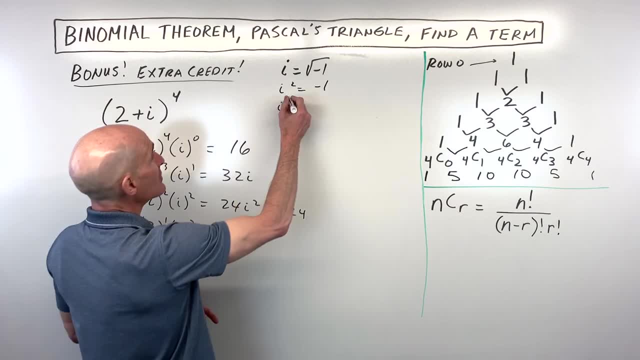 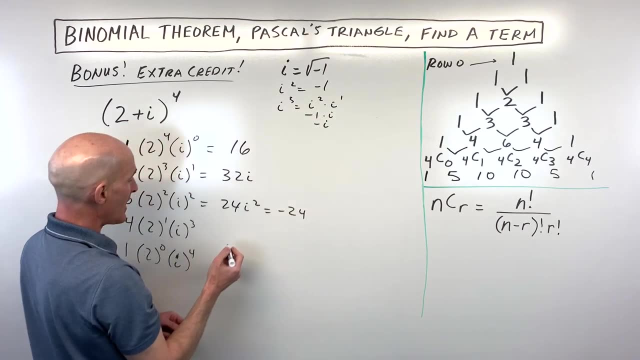 And then i cubed. i cubed is equal to i squared times i, to the first i squared, we know, is negative 1 times i is negative i, So this would be 2 times 4 is 8 times negative i, which would be negative 8i. 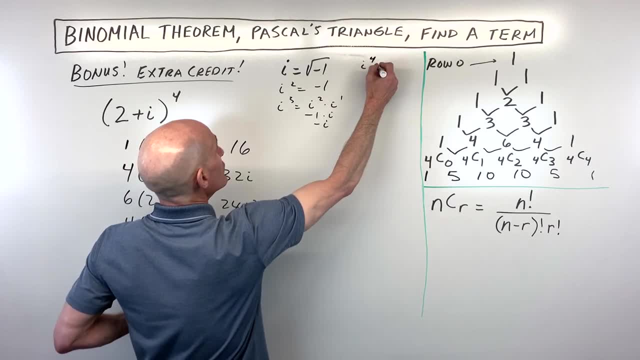 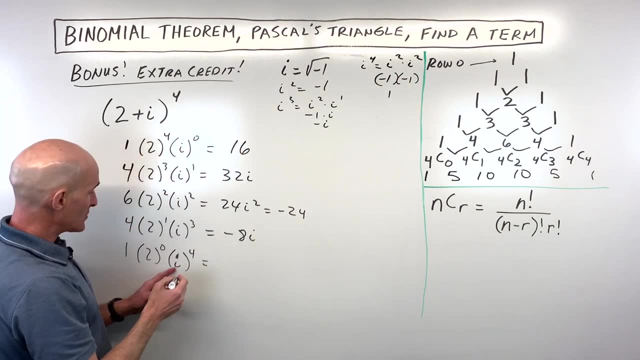 And then over here. i to the fourth is equal to i squared times i squared. i squared is negative 1 times negative 1, which is positive 1.. So this is 2 to the zero is 1.. i to the fourth is 1 times 1 is 1..